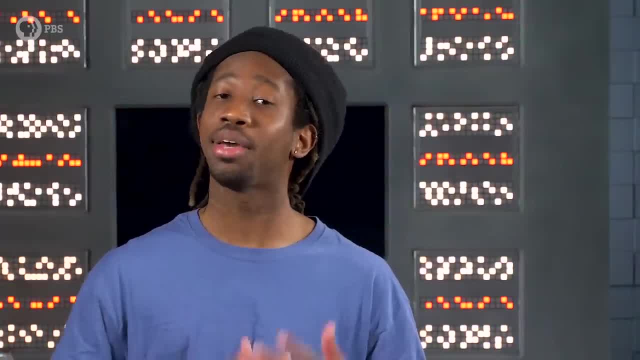 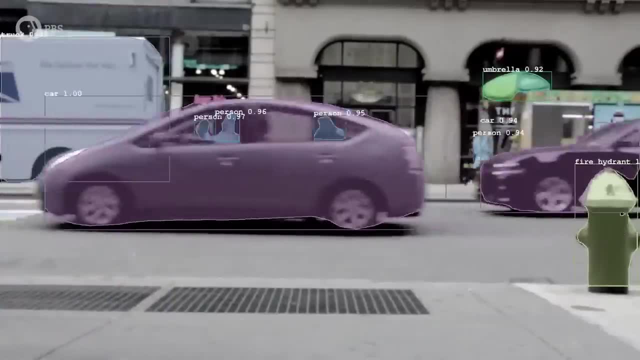 between them. We can actually do a lot more with AI if we connect a bunch of perceptrons together to create what's called an artificial neural network. Neural networks are better than other methods for certain tasks like image recognition. The secret to their success is their hidden layers, and they're mathematically very 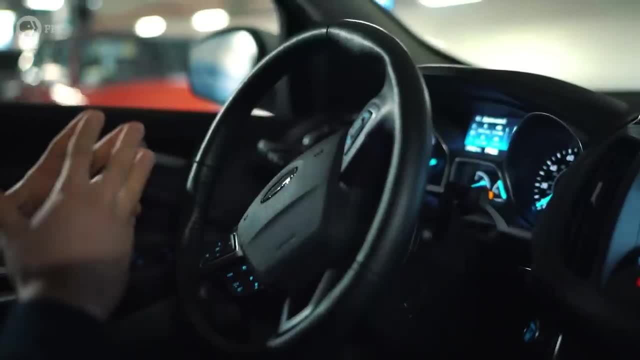 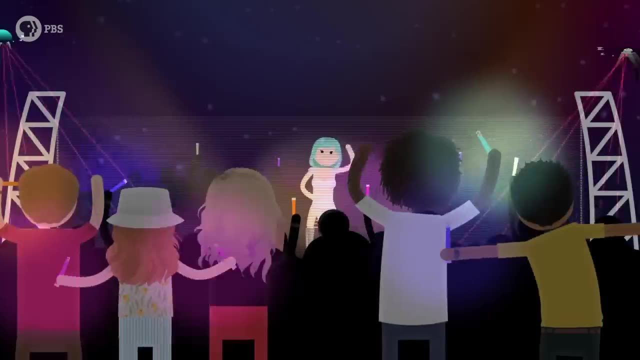 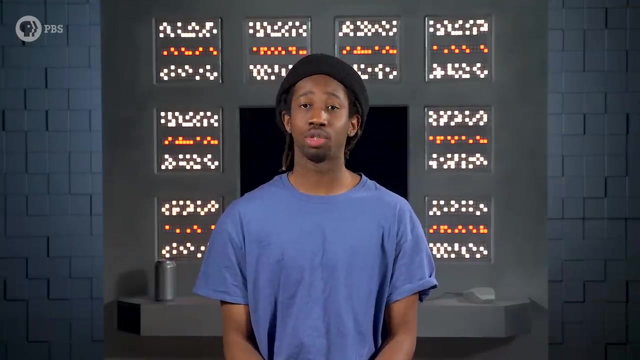 elegant. Both of these are reasons why neural networks are one of the most dominant machine learning technologies used today. Not that long ago, a big challenge in AI was real-world image recognition, like recognizing a dog from a cat, A car from a plane from a boat. 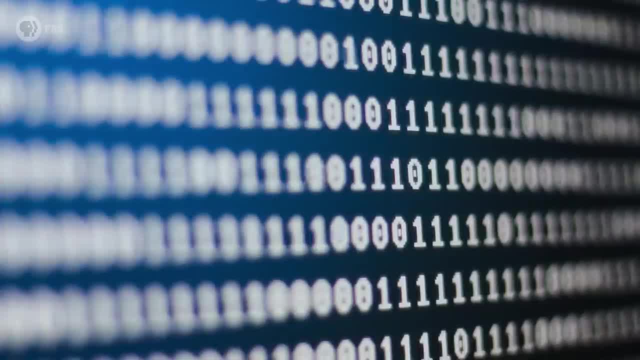 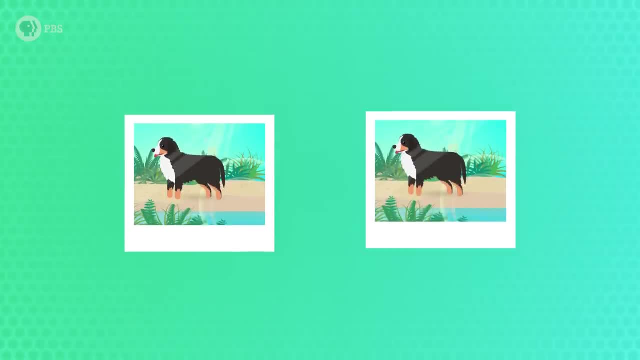 Even though we do it every day, it's really hard for computers. That's because computers are good at literal comparisons like matching zeros and ones one at a time. It's easy for a computer to tell that these images are the same by matching the pixels. 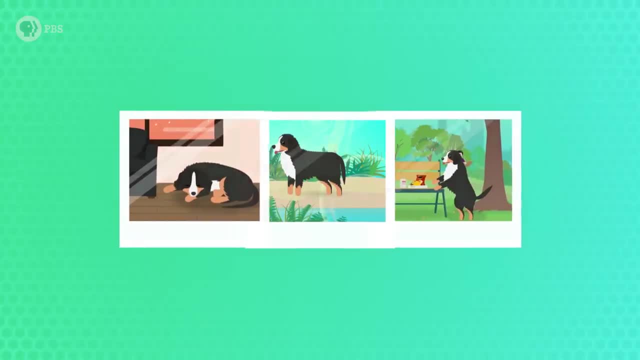 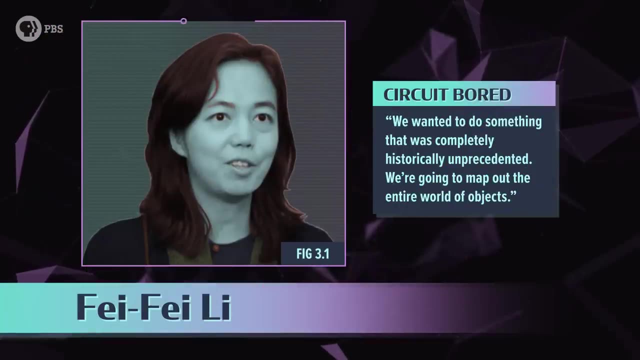 But before AI, a computer couldn't tell that all of these images are of the same dog and had no hope of telling that all of these different images are dogs. So a professor named Fei-Fei Li and a group of other machine learning and computer vision 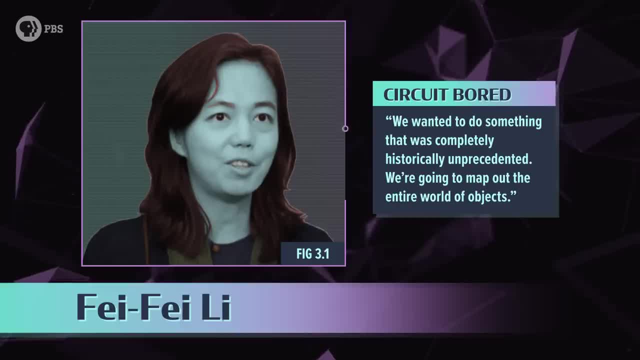 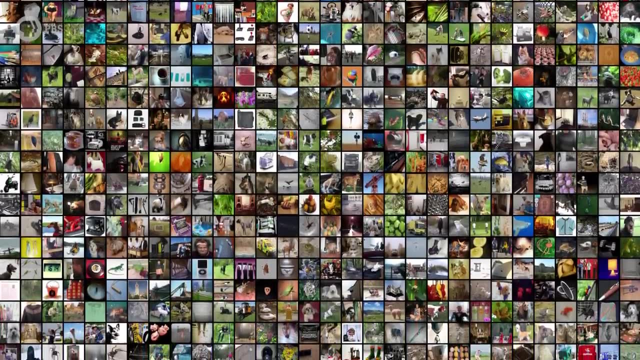 researchers wanted to help the research community develop AI that could recognize images. The first step was to create a huge public dataset of labeled real-world photos. That way, computer scientists around the world could come up with and test different algorithms. They called this dataset ImageNet. 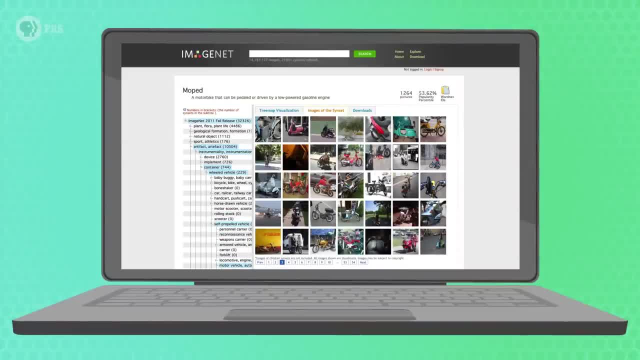 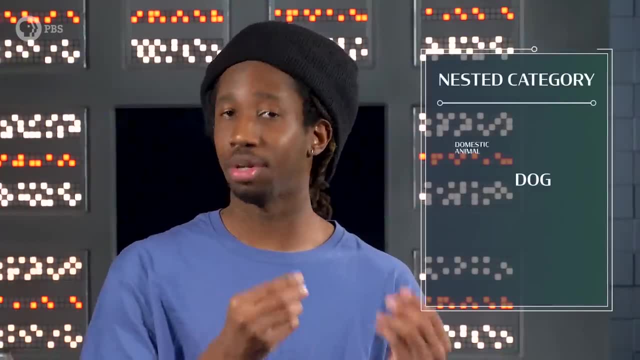 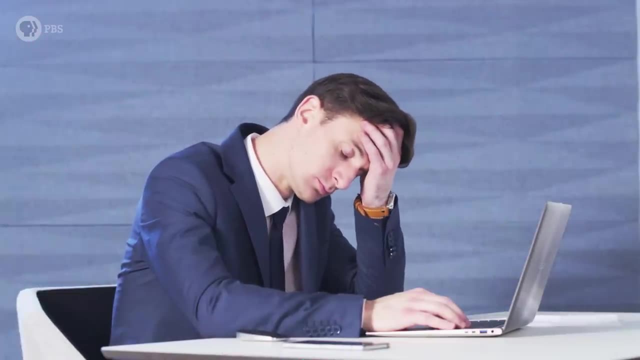 It had 3.2 million labeled images sorted into 5,247 nested categories of nouns, Like, for example: the dog label is nested under domestic animal, which is nested under animal. Humans are the best at reliably labeling data, But if one person did all this labeling, taking 10 seconds per label, without any sleep or 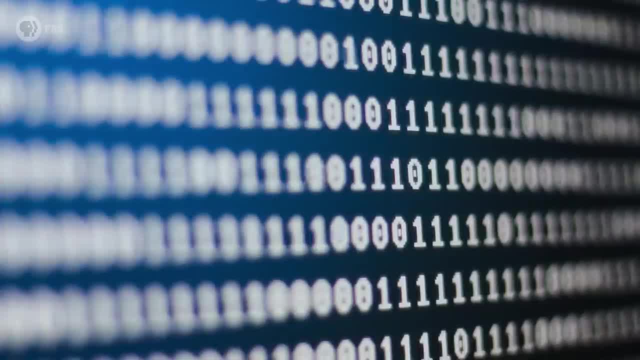 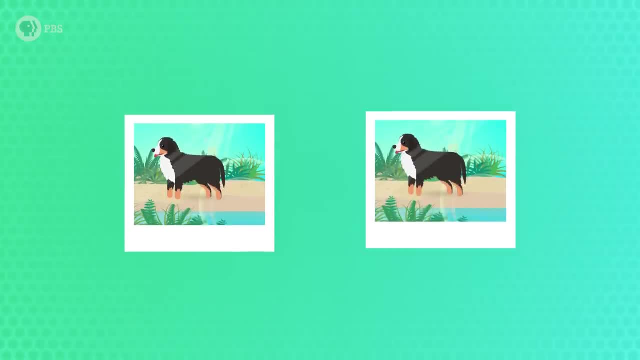 Even though we do it every day, it's really hard for computers. That's because computers are good at literal comparisons like matching zeros and ones one at a time. It's easy for a computer to tell that these images are the same by matching the pixels. 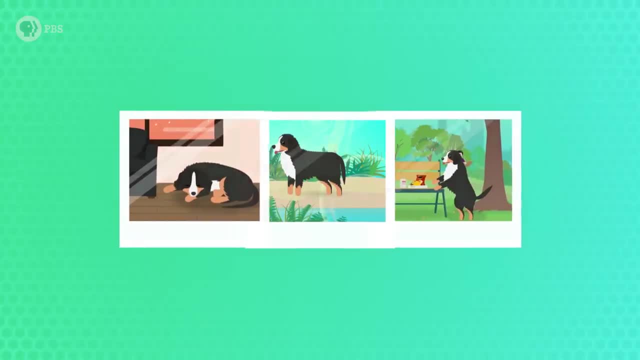 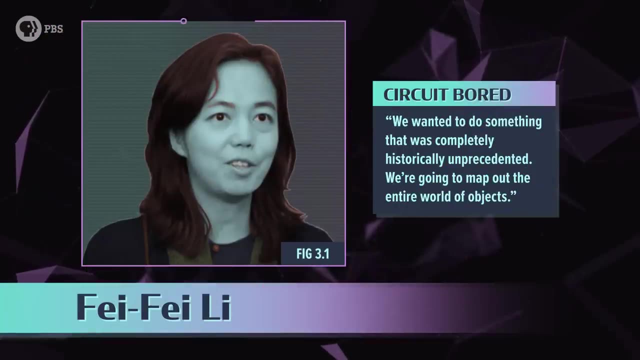 But before AI, a computer couldn't tell that all of these images are of the same dog and had no hope of telling that all of these different images are dogs. So a professor named Fei-Fei Li and a group of other machine learning and computer vision 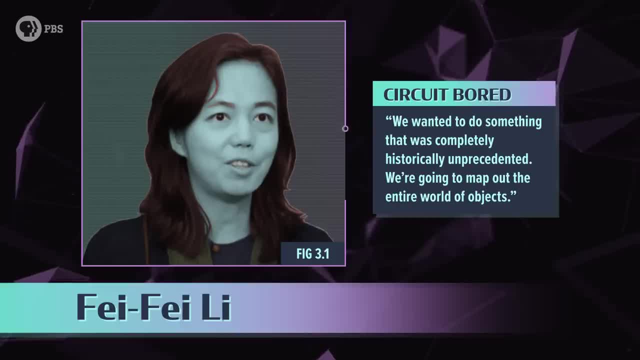 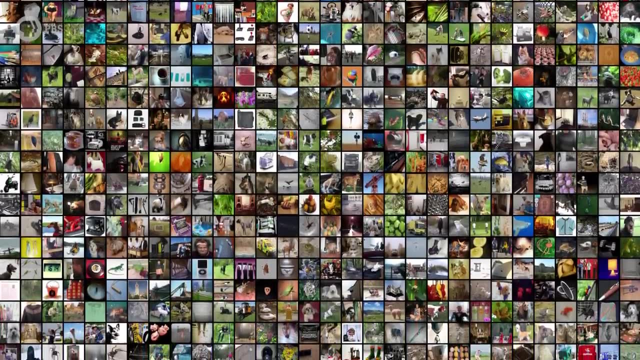 researchers wanted to help the research community develop AI that could recognize images. The first step was to create a huge public dataset of labeled real-world photos. That way, computer scientists around the world could come up with and test different algorithms. They called this dataset ImageNet. 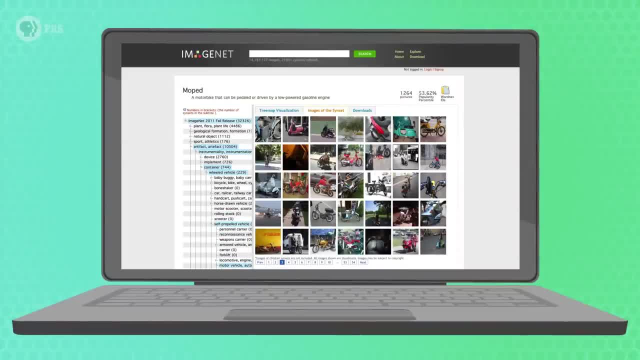 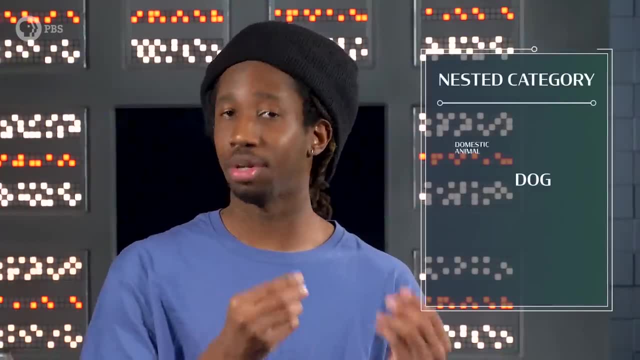 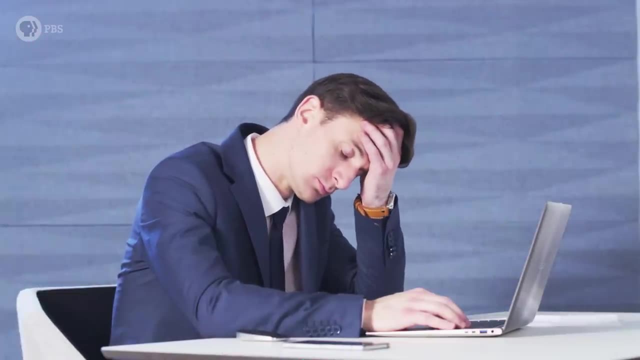 It had 3.2 million labeled images sorted into 5,247 nested categories of nouns, Like, for example: the dog label is nested under domestic animal, which is nested under animal. Humans are the best at reliably labeling data, But if one person did all this labeling, taking 10 seconds per label, without any sleep or 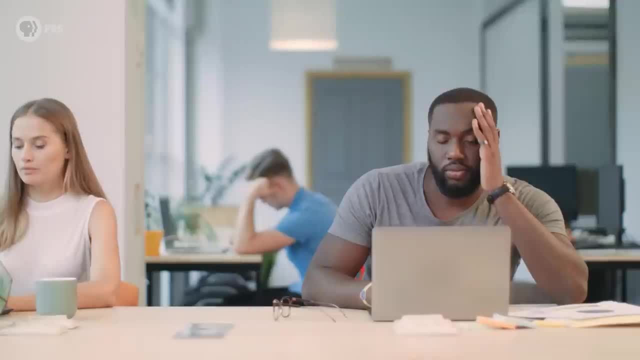 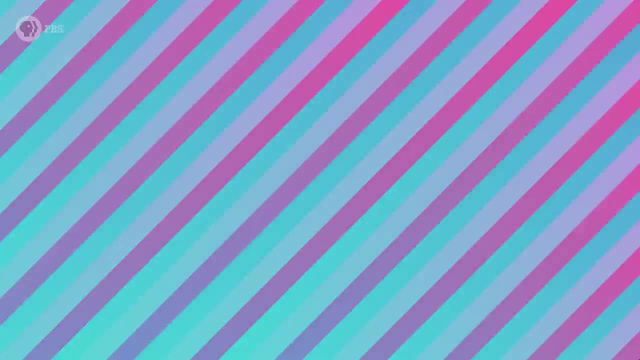 snack breaks. it would take them over a year. So ImageNet used crowdsourcing and leveraged the power of the internet to cheaply spread the work between thousands of people. Once the data was in place, the researchers started an annual competition in 2010 to get 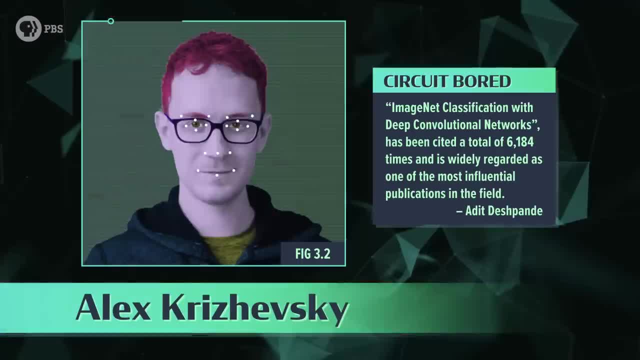 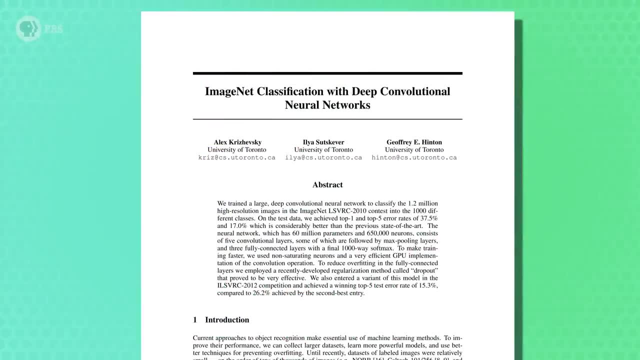 people to contribute their best solutions to image recognition. Enter Alex Krishnan. He was a graduate student at the University of Toronto. In 2012,, he decided to apply a neural network to ImageNet, even though similar solutions hadn't been successful in the past. 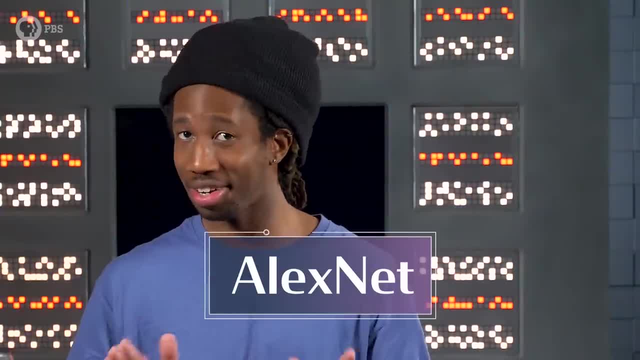 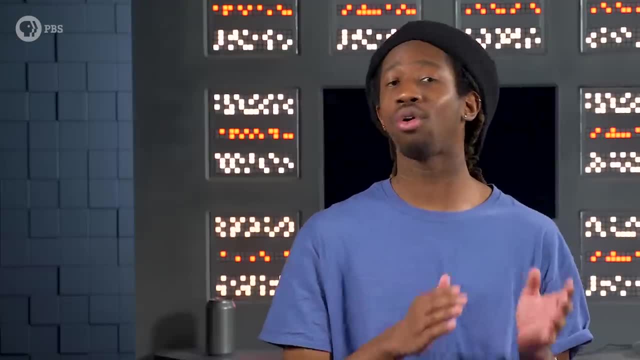 His neural network, called AlexNet, had a couple of innovations that set it apart. He used a lot of hidden layers, which we'll get into in a minute. He also used faster computation hardware to handle all the math that neural networks do. 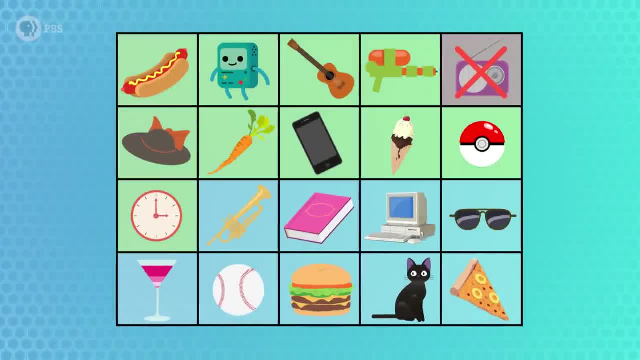 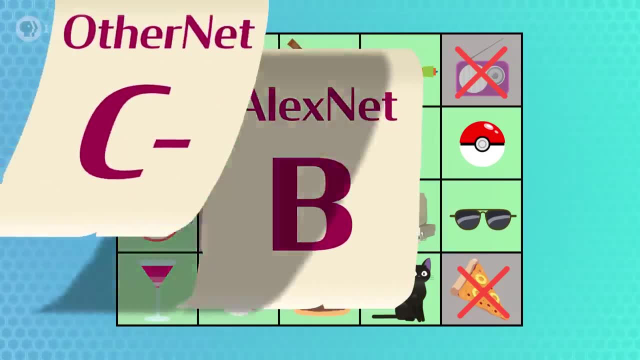 AlexNet outperformed the next best approaches by over 10%. It only got 3 out of 20 images. In grade terms, it was getting a solid B, while other techniques were scraping by with a low C. Since 2012,, neural networks have taken over the annual competition and the results keep. 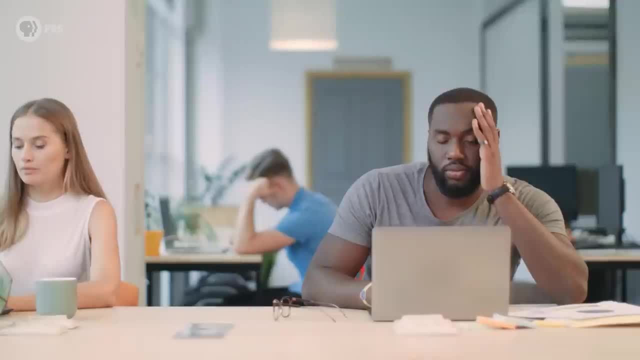 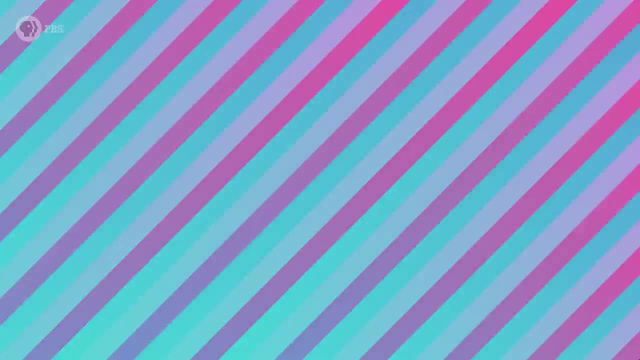 snack breaks. it would take them over a year. So ImageNet used crowdsourcing and leveraged the power of the internet to cheaply spread the work between thousands of people. Once the data was in place, the researchers started an annual competition in 2010 to get 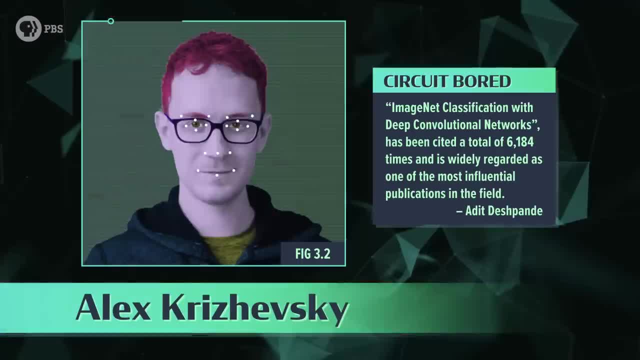 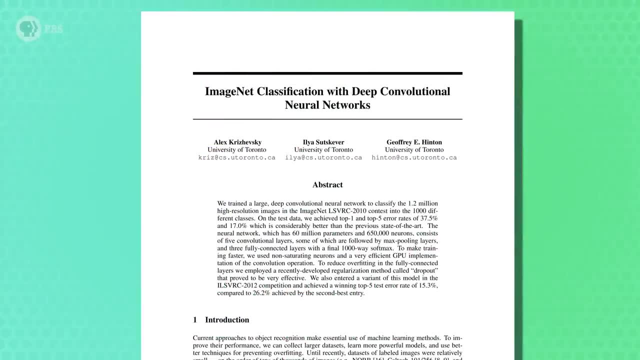 people to contribute their best solutions to image recognition. Enter Alex Krishnan. He was a graduate student at the University of Toronto. In 2012,, he decided to apply a neural network to ImageNet, even though similar solutions hadn't been successful in the past. 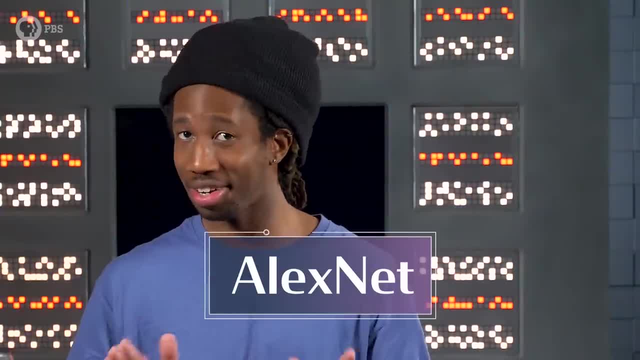 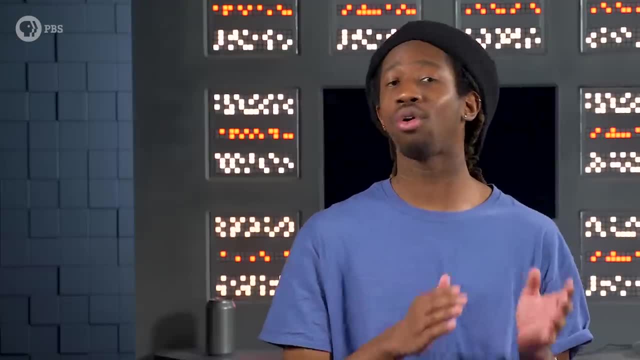 His neural network, called AlexNet, had a couple of innovations that set it apart. He used a lot of hidden layers, which we'll get into in a minute. He also used faster computation hardware to handle all the math that neural networks do. 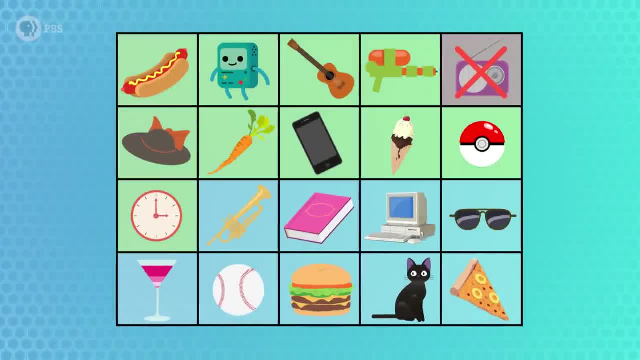 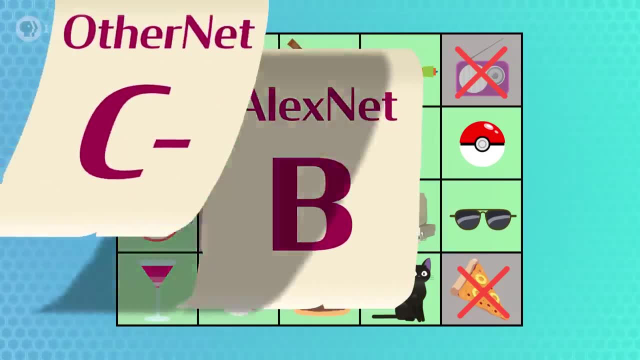 AlexNet outperformed the next best approaches by over 10%. It only got 3 out of 20 images. In grade terms, it was getting a solid B, while other techniques were scraping by with a low C. Since 2012,, neural networks have taken over the annual competition and the results keep. 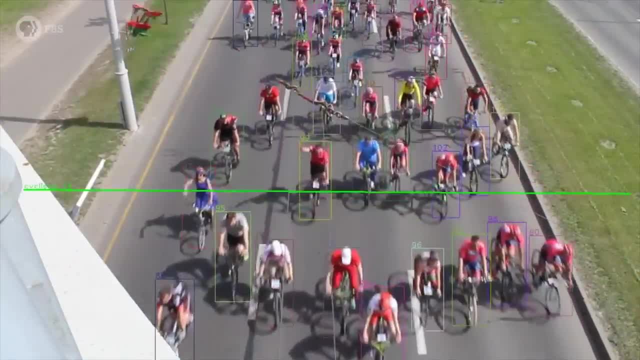 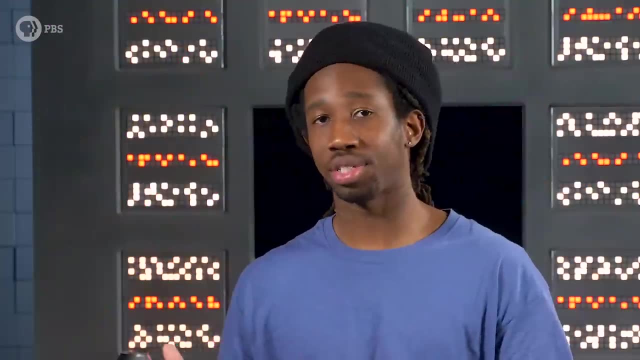 getting better and better. Plus, AlexNet sparked an explosion of research into neural networks, which we started to apply to lots of things beyond image recognition. To understand how neural networks can be used for these classification problems, we have to understand their architecture first. 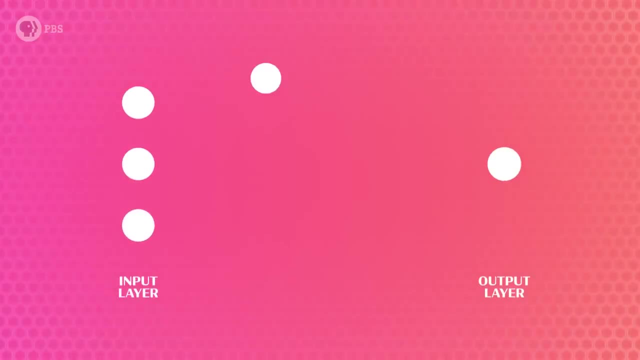 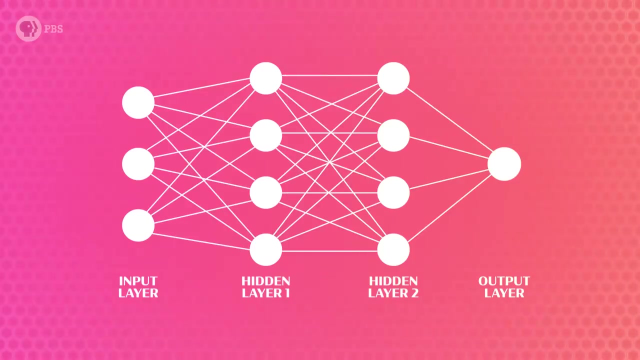 All neural networks are made up of an input layer, an output layer and a number of other layers. There are many different arrangements, but we'll use the classic multi-layer perceptron as an example. The input layer is where the neural network receives data represented as numbers. 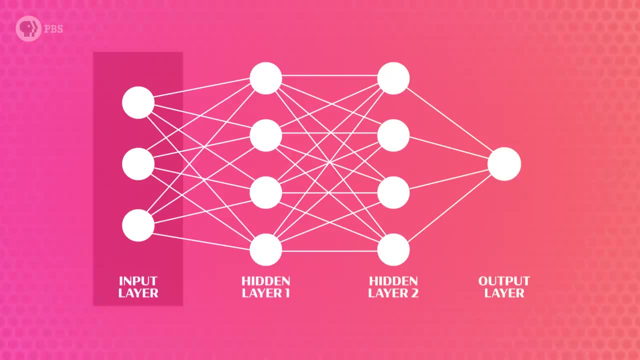 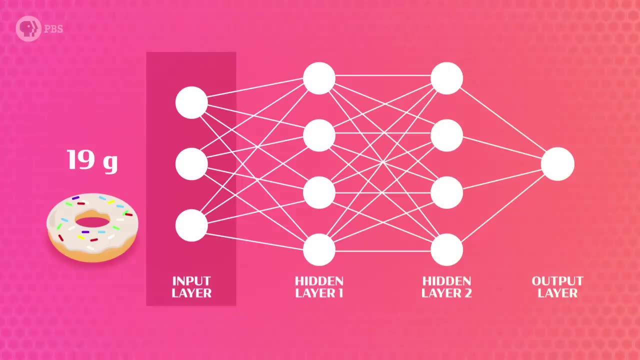 Each input neuron represents a single feature, which is some characteristic of the data. Features are straightforward if you're talking about something that's already a number, like grams of sugar in a donut, But really just about anything can be converted into a number. 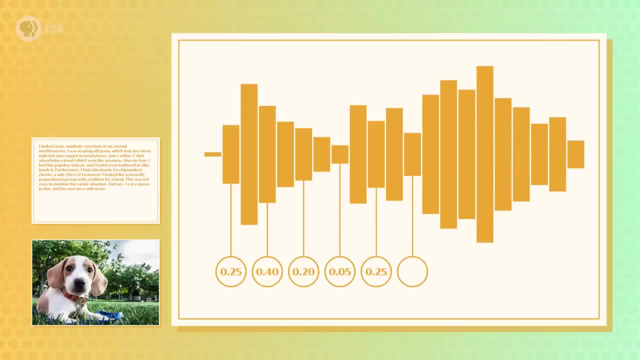 Sounds can be represented as the amplitudes of the sound wave. Sounds can be represented as the amplitudes of the sound wave. Sounds can be represented as the amplitudes of the sound wave, So each feature would have a number that represents the amplitude at a moment in time. 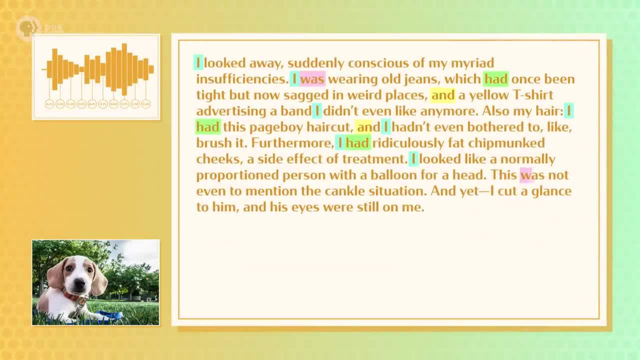 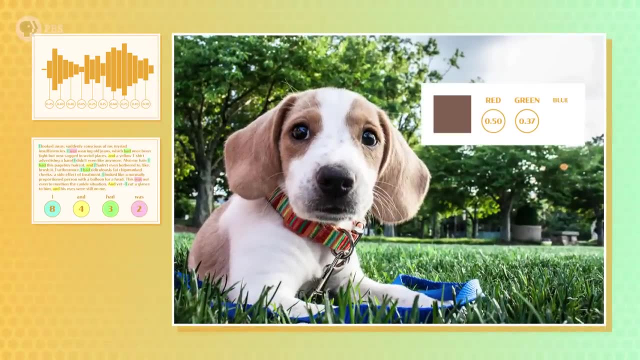 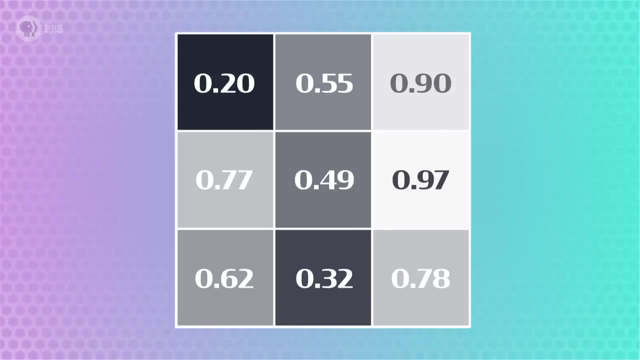 Words in a paragraph can be represented by how many times each word appears. So each feature would have the frequency of one word. Or if we're trying to label an image of a dog, each feature would represent information about a pixel. So for a grayscale image, each feature would have a number representing how bright a pixel. 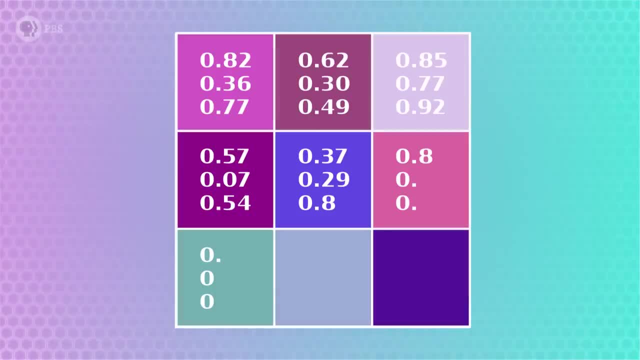 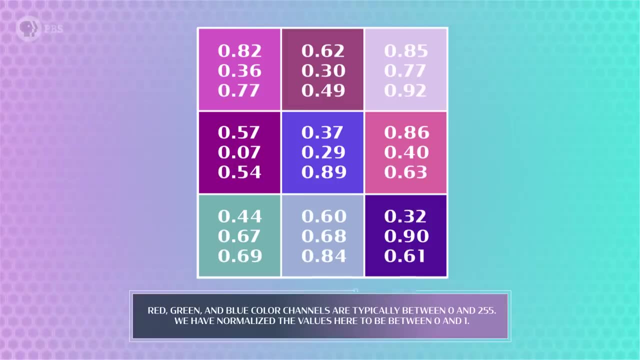 is, But for a color image. we can represent each pixel with three numbers: the amount of red, green and blue which can be combined to make any color on your computer screen. Once the features have data, each one sends its number to every neuron in the next layer. 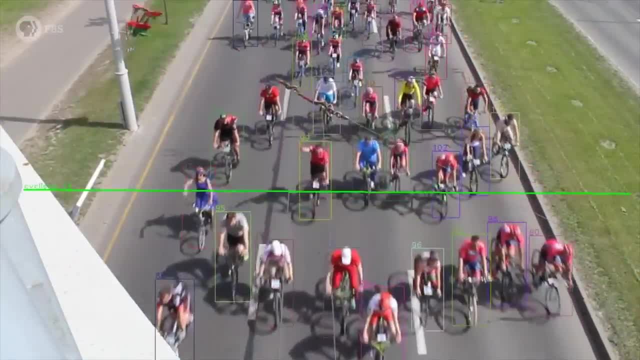 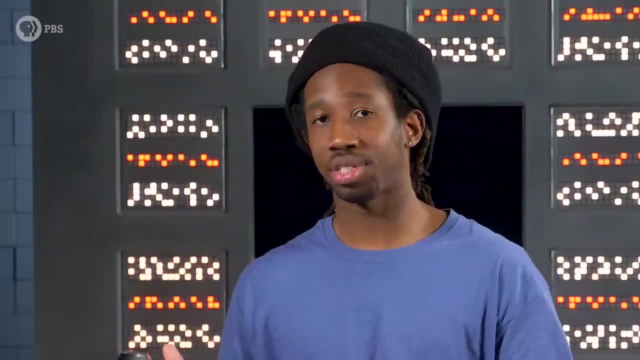 getting better and better. Plus, AlexNet sparked an explosion of research into neural networks, which we started to apply to lots of things beyond image recognition. To understand how neural networks can be used for these classification problems, we have to understand their architecture first. 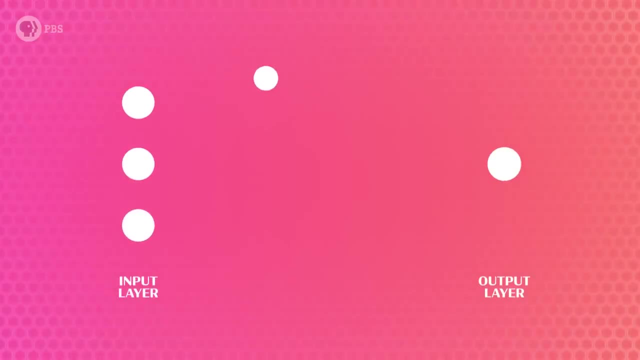 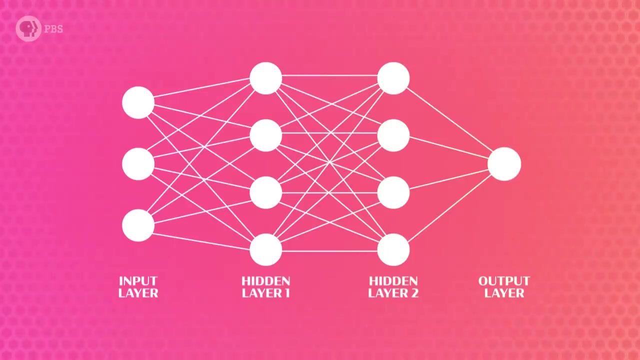 All neural networks are made up of an input layer, an output layer and a number of other layers. All neural networks are made up of an input layer, an output layer and a number of other hidden layers in between. There are many different arrangements, but we'll use the classic multi-layer perceptron. 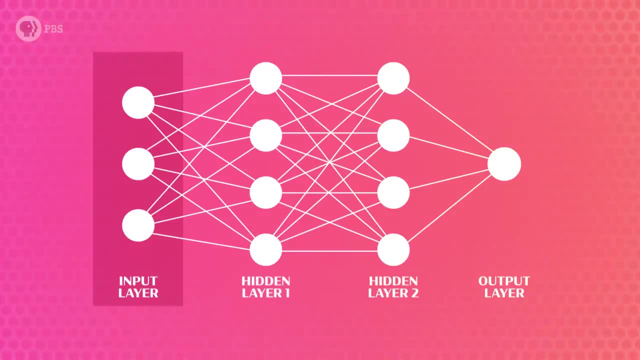 as an example. The input layer is where the neural network receives data represented as numbers. Each input neuron represents a single feature, which is some characteristic of the data. Features are straightforward if you're talking about something that's already a number, like grams of sugar in a donut. 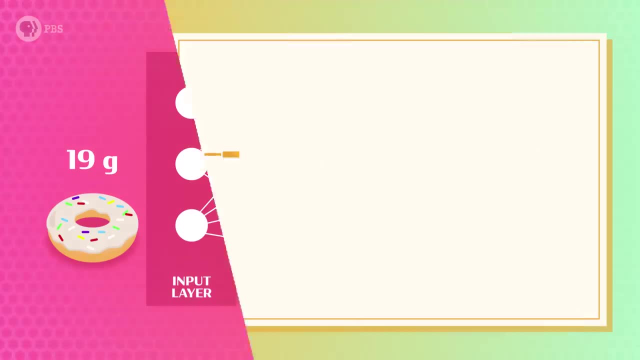 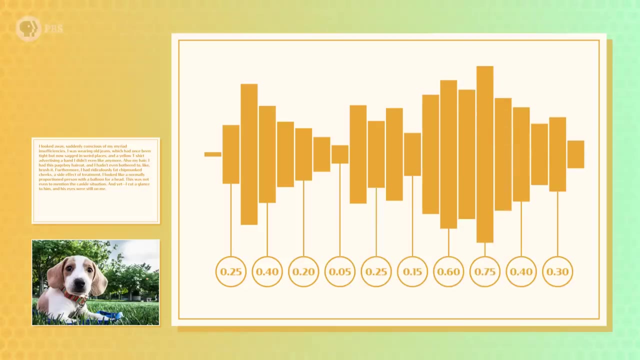 But really just about anything can be converted into a number. Sounds can be represented as the amplitudes of the sound waves. Sounds can be represented as the amplitudes of the sound waves, So each feature would have a number that represents the amplitude at a moment in time. 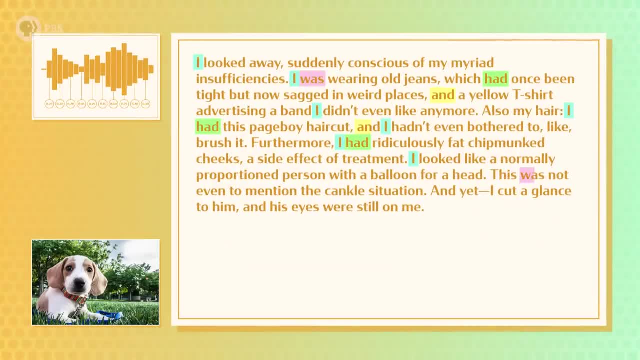 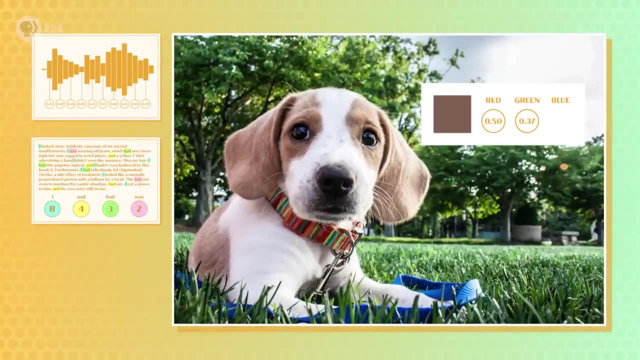 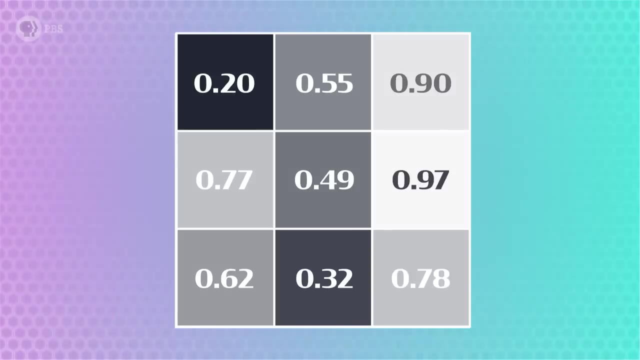 Words in the paragraph can be represented by how many times each word appears. So each feature would have the frequency of one word. Or if we're trying to label an image of a dog, each feature would represent information about a pixel. So for a grayscale image, each feature would have a number representing how bright a pixel. 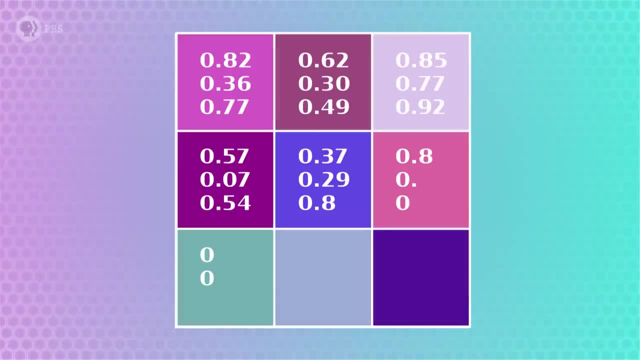 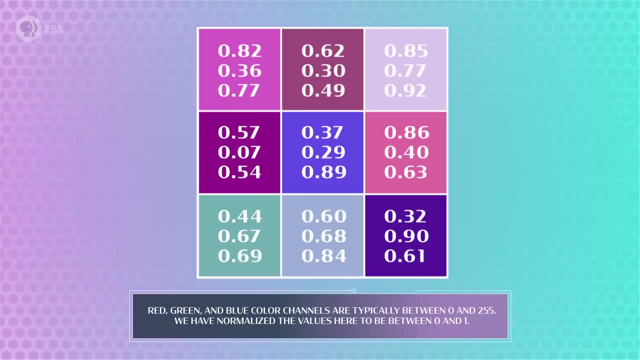 is, But for a color image. we can represent each pixel with three numbers: The amount of red, green and blue Which can be combined to make any color on your computer screen. Once the features have data, each one sends its number to every neuron in the next layer. 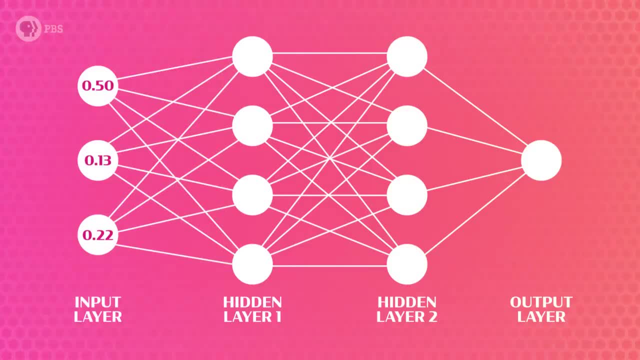 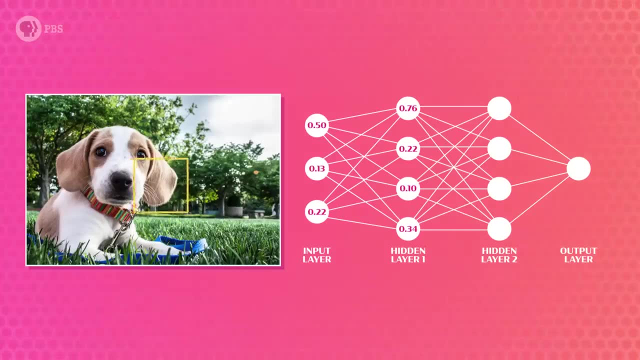 called the hidden layer. Then each hidden layer neuron mathematically combines all the numbers it gets. The goal is to measure whether the input data has certain components For an image recognition problem. these components may be a certain color in the center, a curve. 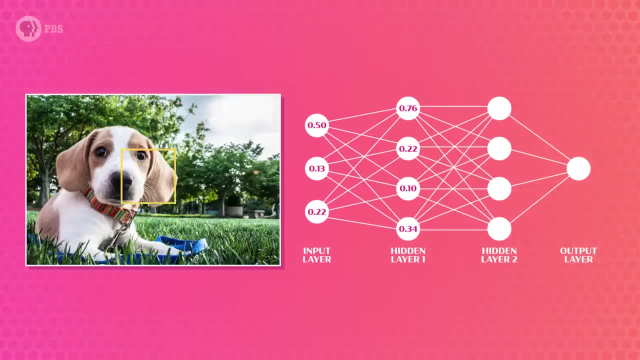 near the top, Or even whether the image contains eyes, Ears Or fur. Instead of answering yes or no, like the simple perceptron from the previous episode, each neuron in the hidden layer does some slightly more complicated math and outputs a number. 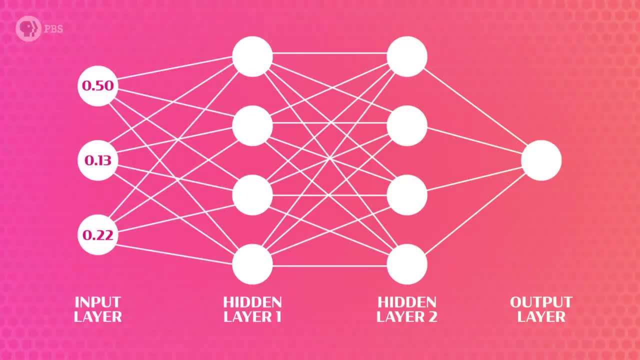 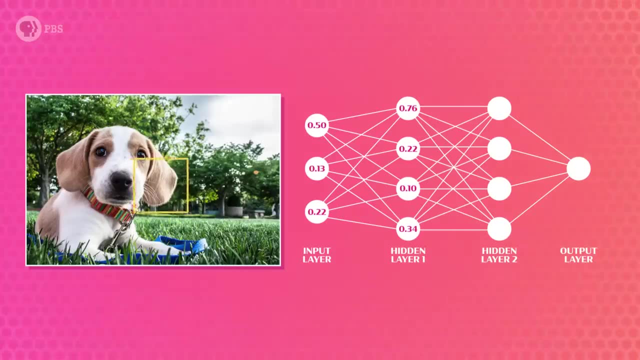 called the hidden layer. Then each hidden layer neuron mathematically combines all the numbers it gets. The goal is to measure whether the input data has certain components For an image recognition problem. these components may be a certain color in the center, a curve. 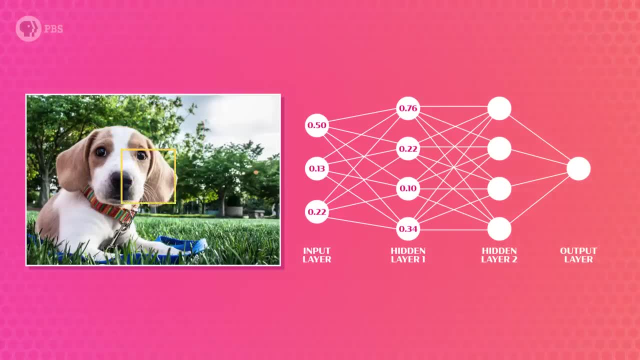 near the top, or even whether the image contains eyes, ears or fur. Instead of answering yes or no, like the simple perceptron from the previous episode, each neuron in the hidden layer does some slightly more complicated math and outputs a number. 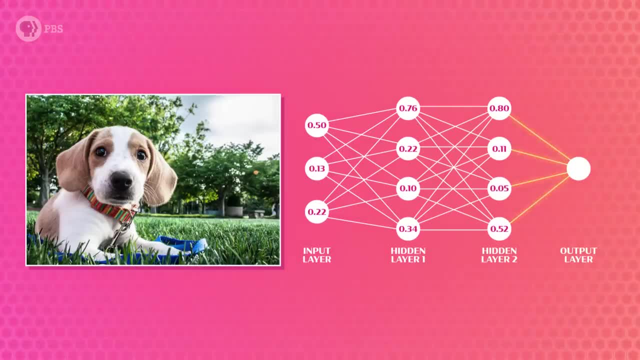 And then each neuron sends its number to every neuron in the next layer, which could be another hidden layer or the output layer. The output layer is where the final hidden layer outputs are mathematically combined to answer the problem. So let's say we're trying to label an image as a dog. 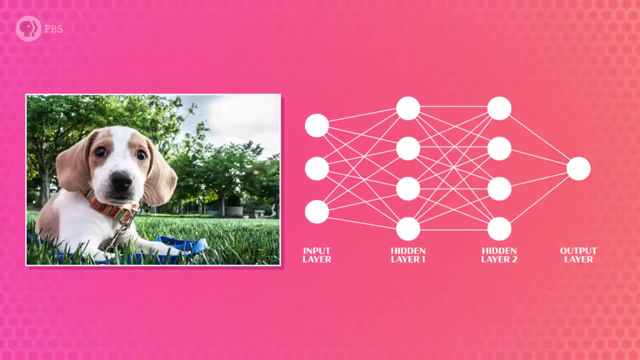 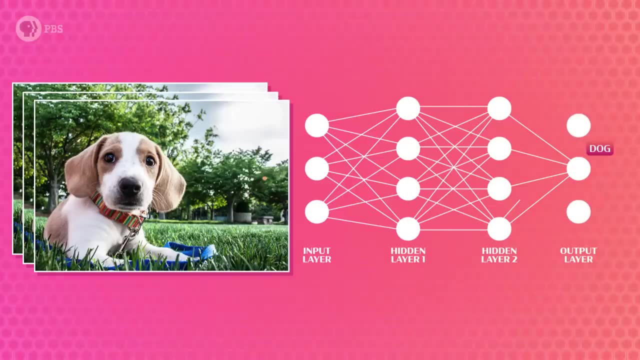 We might have a single output neuron representing a cell. We might have a single answer, that the image is of a dog or not. But if there are many answers- like, for example, if we're labeling a bunch of images- we'll need a lot of output neurons. 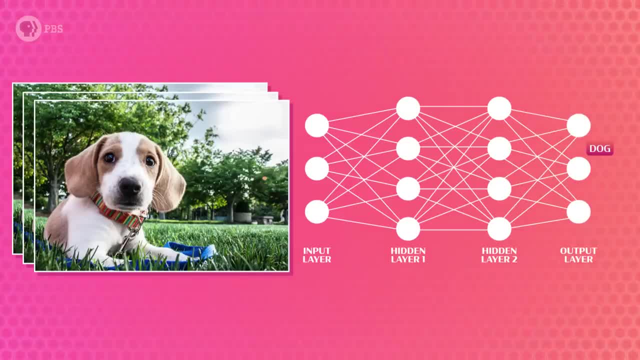 Each output neuron will correspond to the probability for each label, Like, for example, dog, car, spaghetti and more, And then we pick the answer with the highest probability. The key to neural networks and really all of AI, is math. 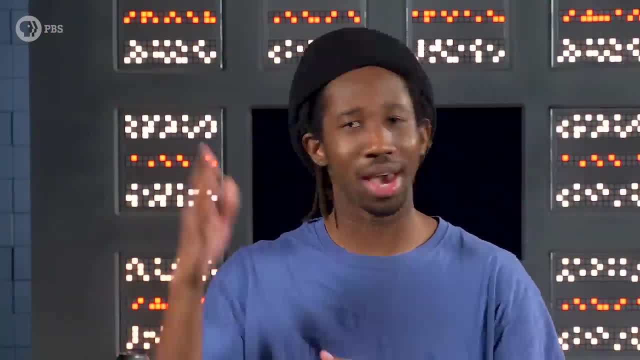 And I get it- A neural network kind of seems like a black box that does math and spits out numbers. But it's not. It's a machine, It's an answer. I mean, those middle layers are even called hidden layers. 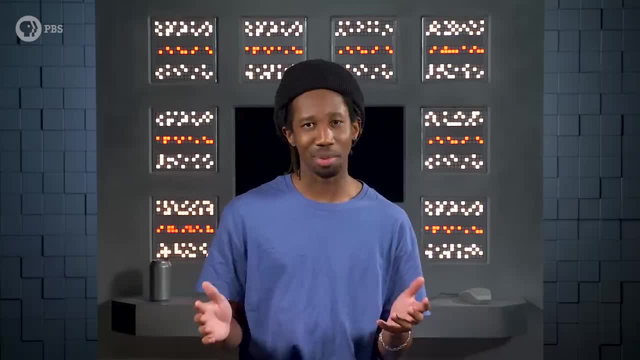 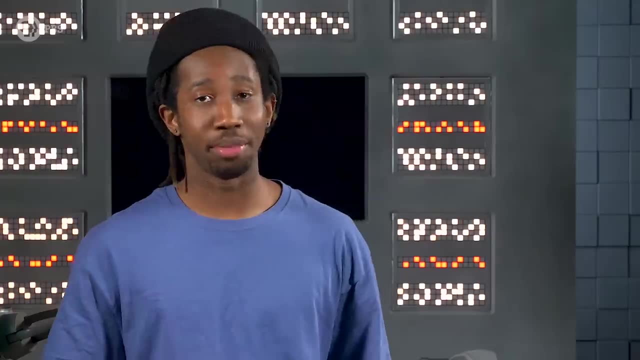 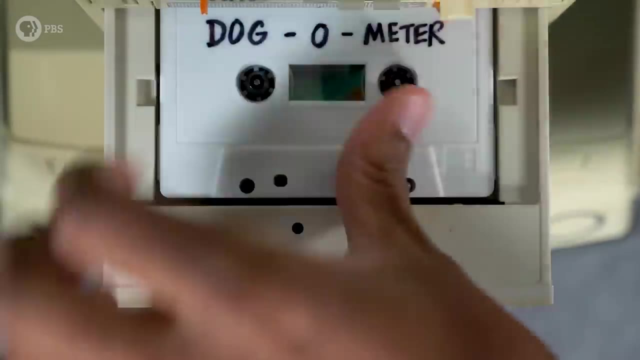 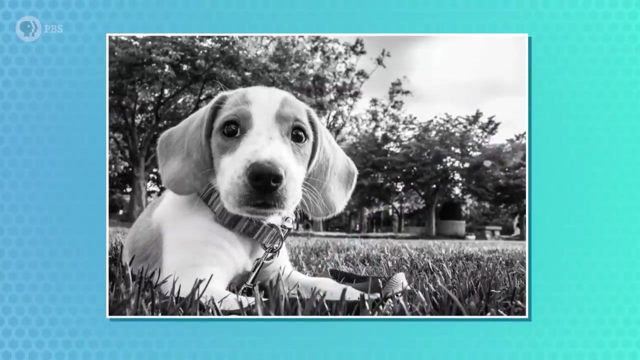 But we can understand the gist of what's happening by working through an example. Oh, John Green Bot. Let's give John Green Bot a program with a neural network that's been trained to recognize a dog in a grayscale photo. When we show him this photo first. 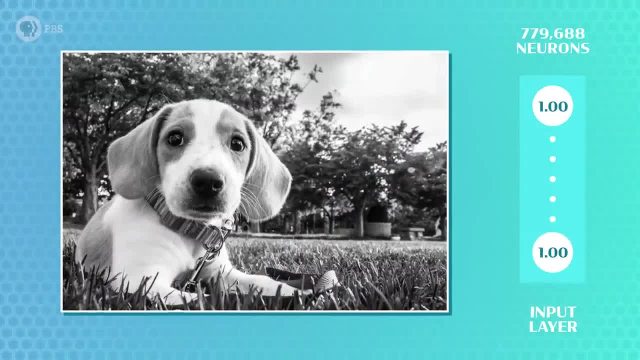 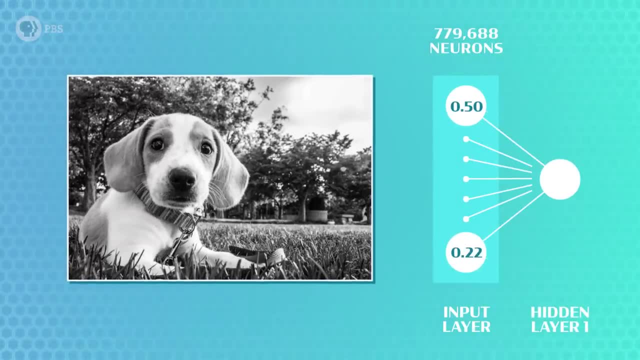 Each feature will contain a number between zero and one, corresponding to the brightness of one pixel, And it'll pass this information to the hidden layer. Now let's focus on one hidden layer: neuron. Since the neural network is already trained. this neuron has a mathematical formula to: 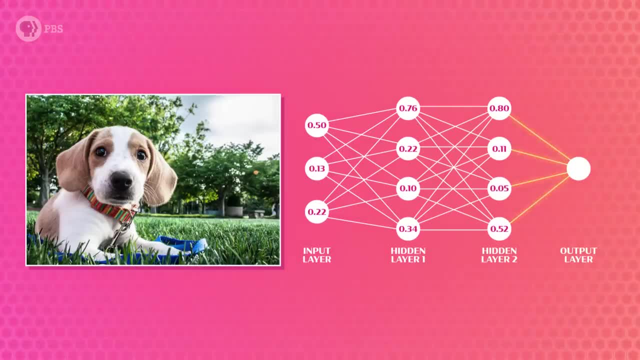 And then each neuron sends its number to every neuron in the next layer, which could be another hidden layer or the output layer. The output layer is where the final hidden layer outputs are mathematically combined to answer the problem. So let's say we're trying to label an image as a dog. 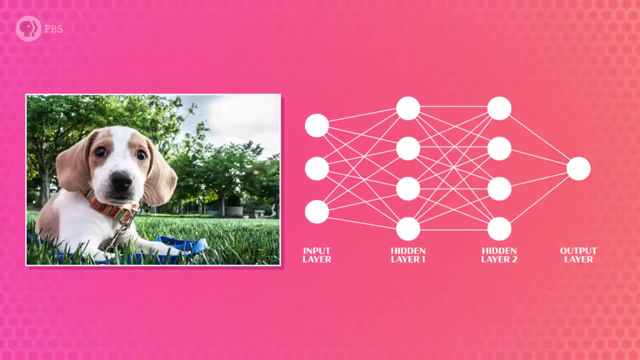 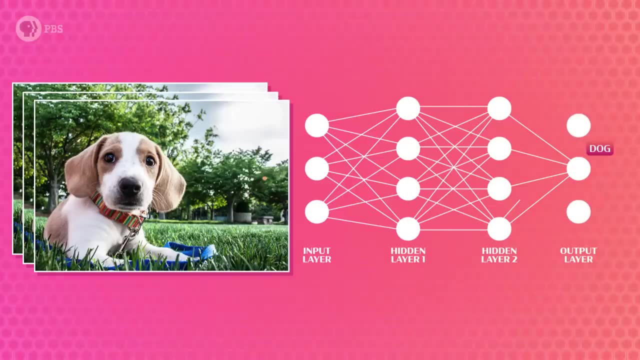 We might have a single output neuron representing a single answer- that the image is of a dog or not. But if there are many answers- like, for example, if we're labeling a bunch of images- we'll need a lot of output neurons. 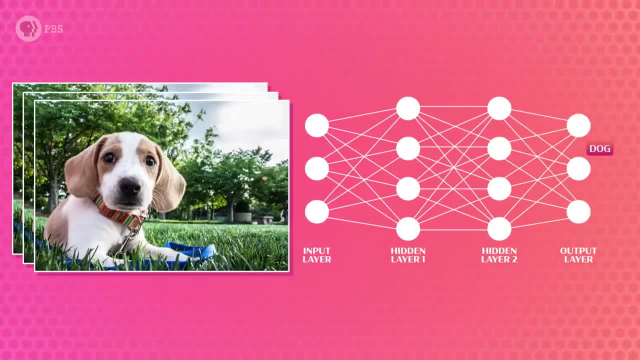 Each output neuron will correspond to the probability for each label, Like, for example, dog, car, spaghetti and more, And then we pick the answer with the highest probability. The key to neural networks and really all of AI, is math. 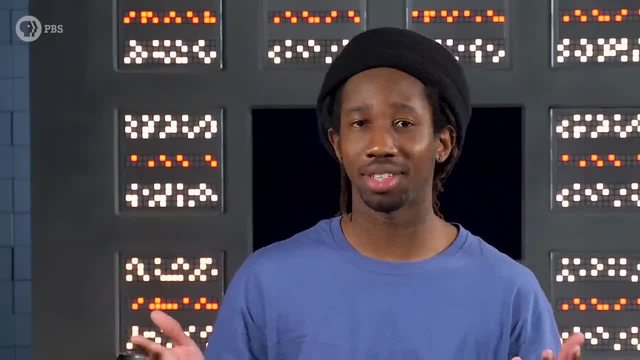 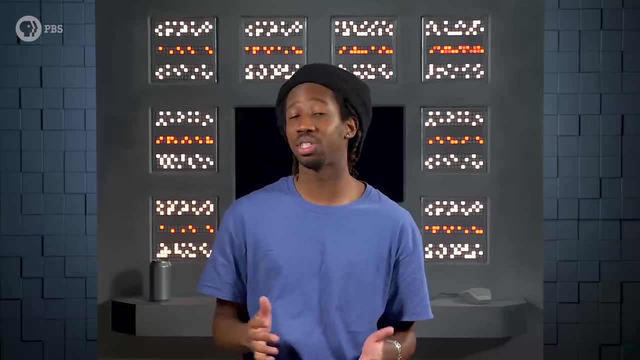 And I get it. I get it. The word kind of seems like a black box that does math and spits out an answer. I mean, those middle layers are even called hidden layers. But we can understand the gist of what's happening by working through an example. 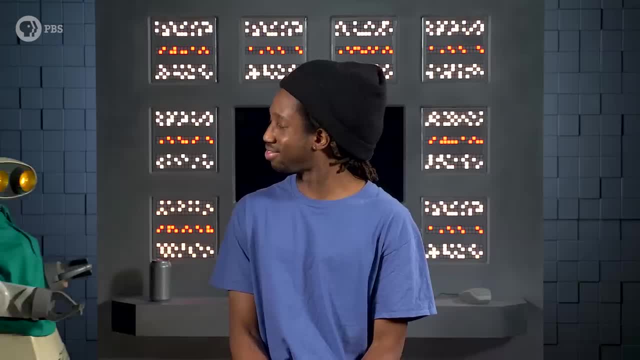 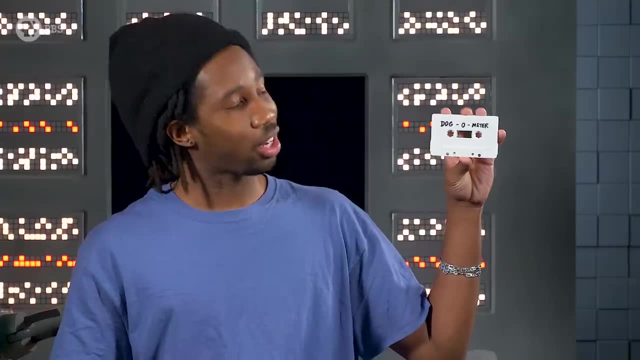 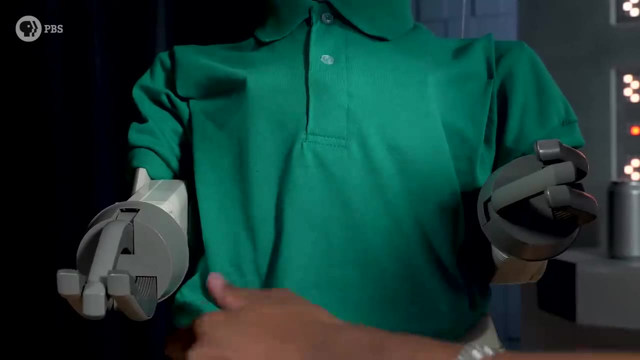 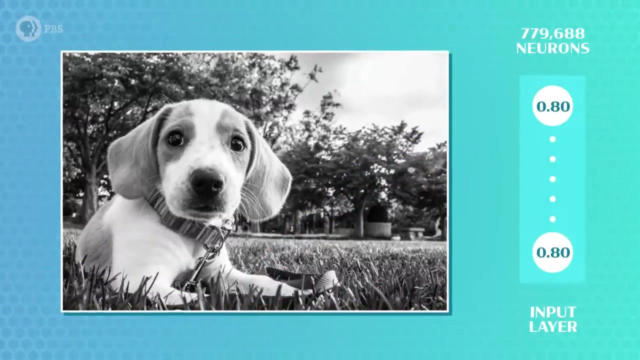 Oh, John Green Bot. let's give John Green Bot a program with a neural network that's been trained to recognize a dog in a grayscale photo When we show him this photo first. each feature will contain a number between 0 and 1, corresponding. 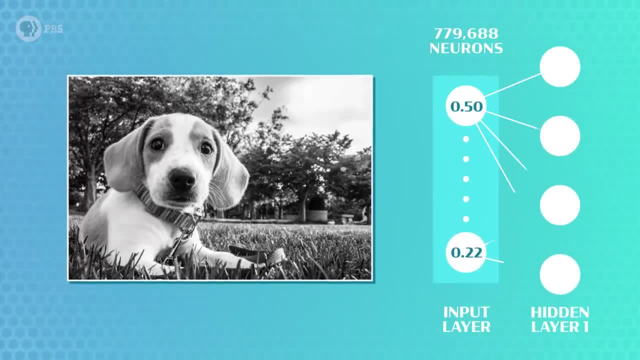 to the brightness of one pixel And it'll pass this information to the hidden layer. Now let's focus on one hidden layer: neuron, Since the neural network is already trained. this neuron has a mathematical formula to look at a particular component in the image. 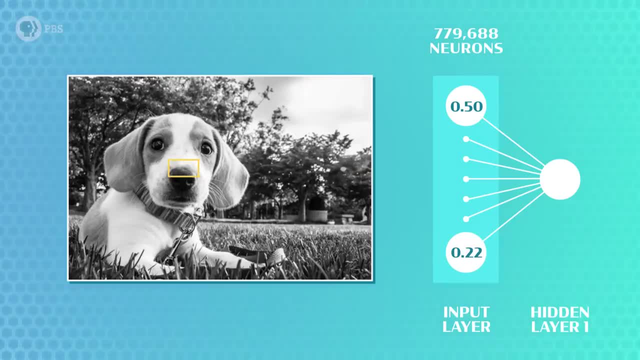 Like a specific curve in the center, The curve at the top of the nose. If this neuron is focused on this specific shape or spot, it may not be able to recognize the dog, But it may not really care what's happening anywhere else. 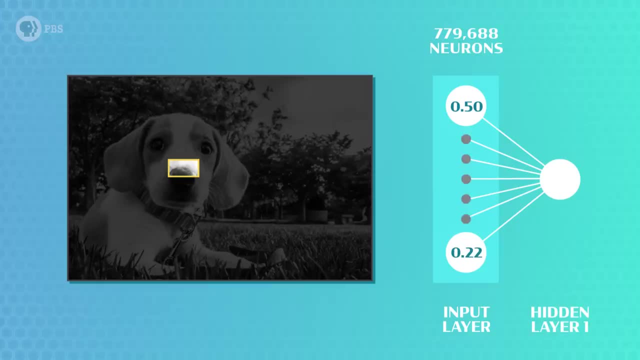 So it would multiply or weigh the pixel values from most of these features by 0, or close to 0. Because it's looking for bright pixels here, it would multiply these pixel values by a positive weight. This curve is also defined by a darker part below. 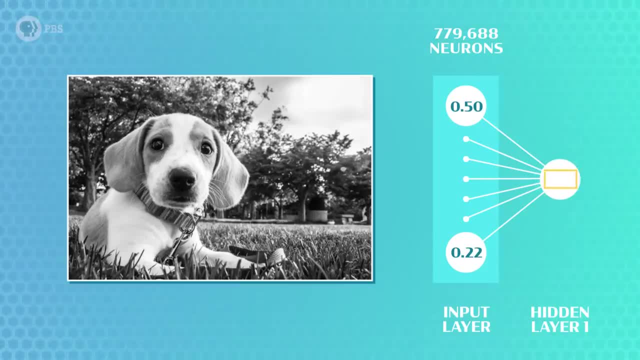 look at a particular component in the image, Like a specific curve in the center, The curve at the top of the nose. If this neuron is focused on this specific shape or spot, it may not really care what's happening anywhere else. So let's take a look. 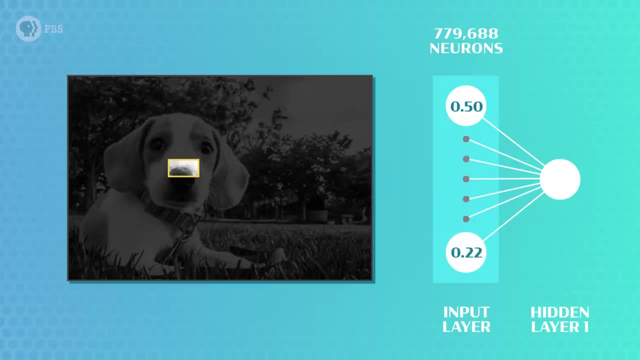 So it would multiply or weigh the pixel values from most of these features by zero Or close to zero. Because it's looking for bright pixels here, it would multiply these pixel values by a positive weight. This curve is also defined by a darker part below. 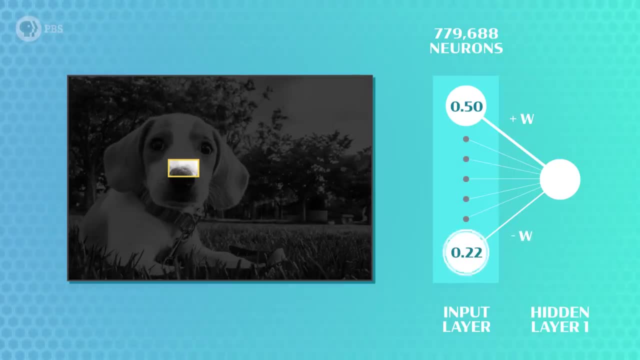 So the neuron will multiply these pixel values by a negative weight. This hidden neuron will add all the weighted pixel values from the input neurons and squish the result so that it's between zero and one. The final number basically represents the guess of this feature. 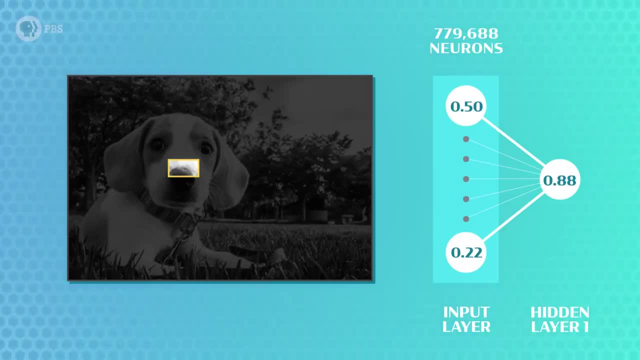 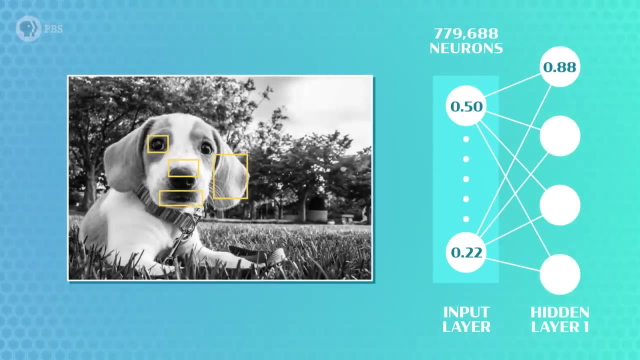 So let's take a look at another example of this neuron thinking that a specific curve, aka a dog nose, appeared in the image. Other hidden neurons are looking for other components, Like, for example, a different curve in another part of the image or a fuzzy texture. 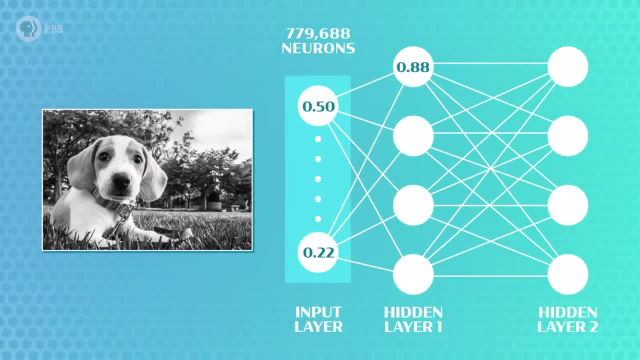 When all of these neurons pass their estimate onto the next hidden layer, those neurons may be trained to look for more complex components. Like one hidden neuron may check whether there's a shape that might be a dog nose, It probably doesn't care about data from previous layers that looked for furry textures. 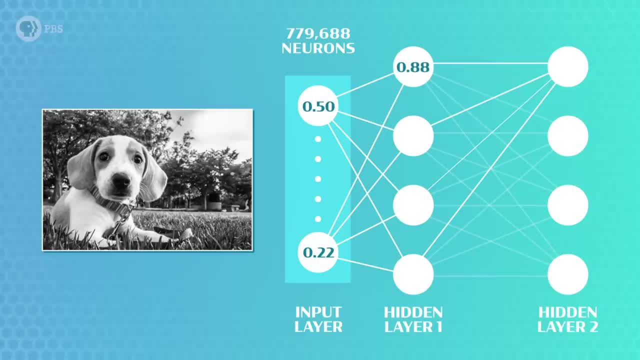 So it weighs those by zero or close to zero. But it may really care about neurons that looked for the top of the nose and the bottom of the nose and nostrils. It weighs those by large positive numbers. Again, it would add up all the weighted values from the previous layer. neurons squish the. 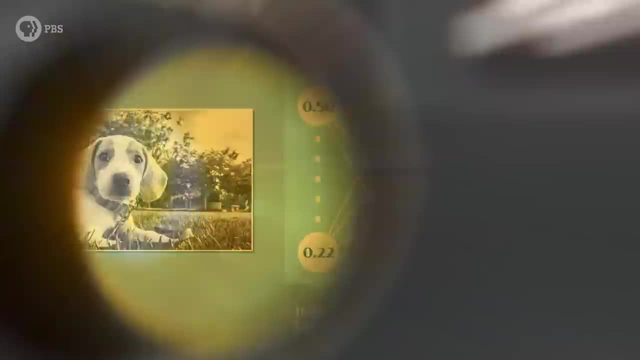 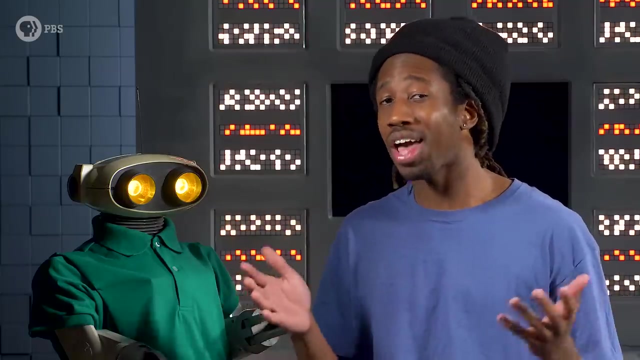 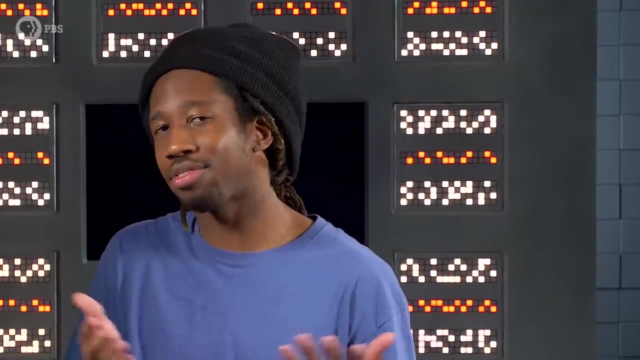 value between zero and one and pass this to the next layer. That's the gist of the math, but we're simplifying it a bit. It's important to know that neural networks don't actually understand ideas like nose or eyelid. Each neuron is doing a calculation on the data it's given and just flagging specific. 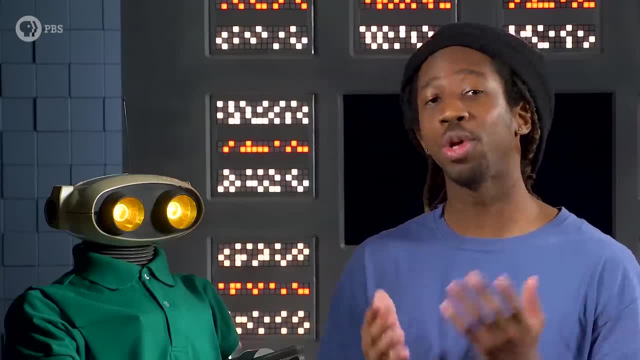 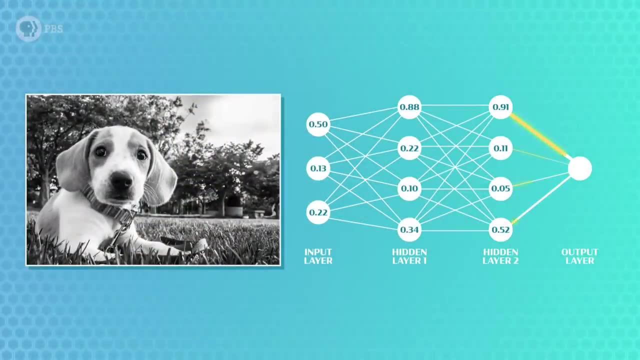 patterns of light and dark. After a few more hidden layers we reach the output layer with one neuron. So after one more weighted addition of the previous layer's data, which happens in the output neuron, the network should have a good estimate if this image is a dog. 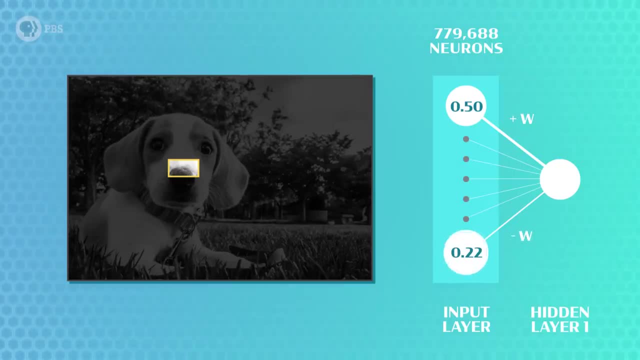 So the neuron will multiply these pixel values by a negative weight. This hidden neuron will add all the weighted pixel values from the input neurons and squish the result. The final number basically represents the guess of this neuron thinking that a specific curve, aka a dog nose, appeared in the image. 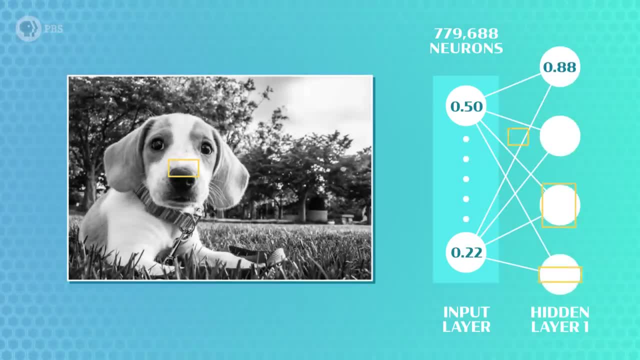 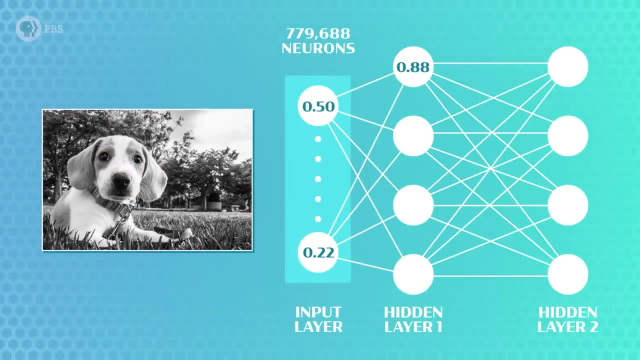 Other hidden neurons are looking for other components Like, for example, a different curve in another part of the image or a fuzzy texture. When all of these neurons pass their estimate onto the next hidden layer, those neurons may be trained to look for more complex components. 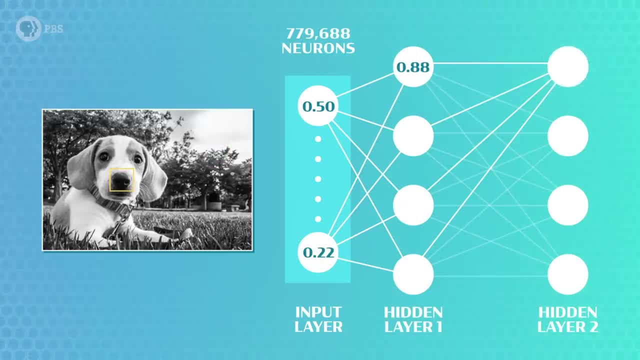 Like one hidden neuron, may check whether there's a shape that might be a dog nose. It probably doesn't care about data from previous layers that looked for furry textures, So it weighs those by 0, or close to 0. But it may really care about neurons that looked for the top of the nose and the bottom. 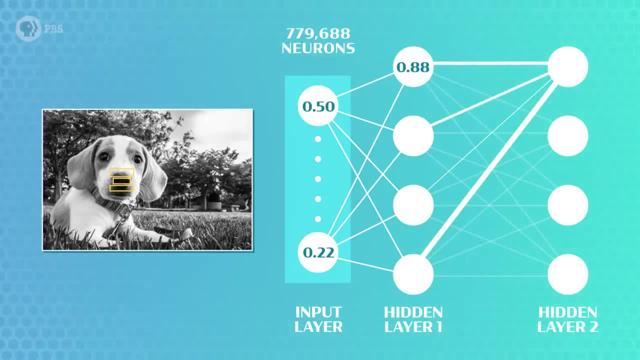 of the nose and nostrils. It weighs those by large positive numbers. Again, it would add up all the weighted values from the previous layer. neurons squish the value between 0 and 1, and pass this to the next layer. 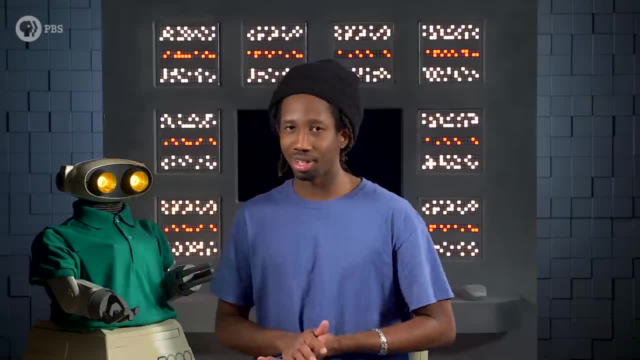 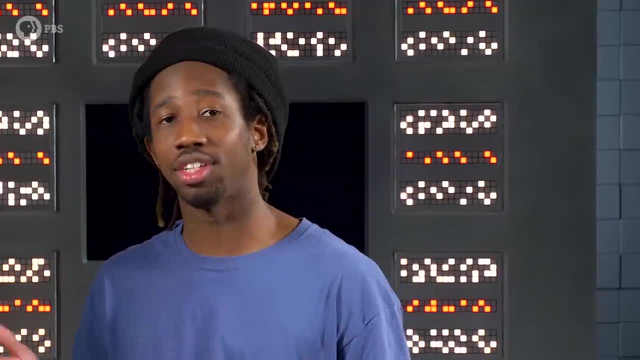 That's the gist of the math, but we're simplifying it a bit. It's important to know that neural networks don't actually understand ideas like nose or eyelid. Each neuron is doing a calculation on the data it's given and just flagging specific. 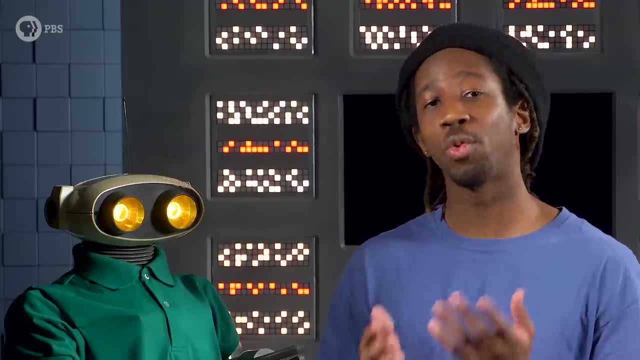 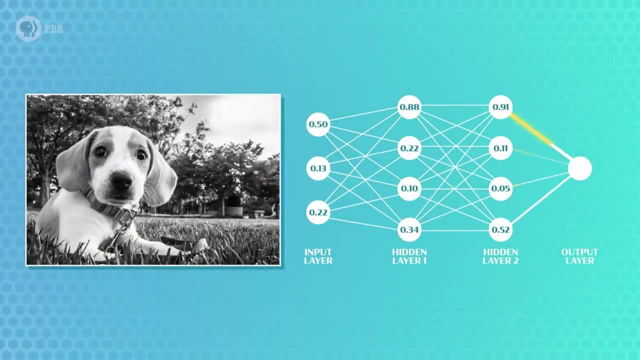 patterns of light and dark. After a few more hidden layers we reach the output layer with one neuron. So after one more weighted addition of the previous layer's data, which happens in the output neuron, the network should have a good estimate if this image is a dog. 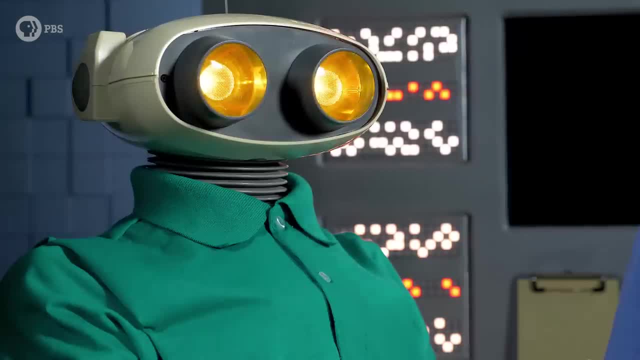 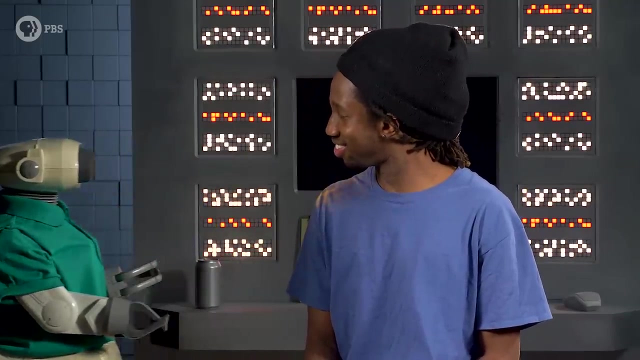 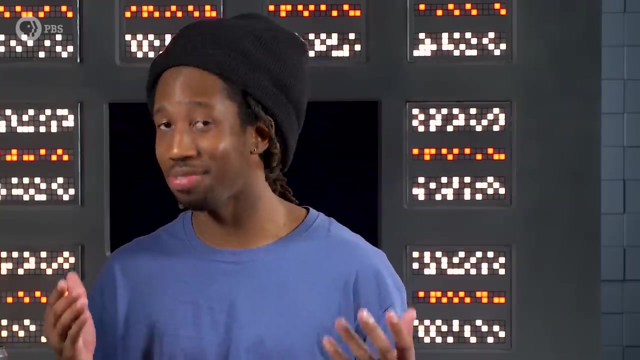 Which means John Greenbot should have a decision. Outro. Hey, John Greenbot, nice job. Thinking about how neural networks would process just one image makes it clearer why AI needs fast computers. Like I mentioned before, each pixel in a color image would be represented by three numbers. 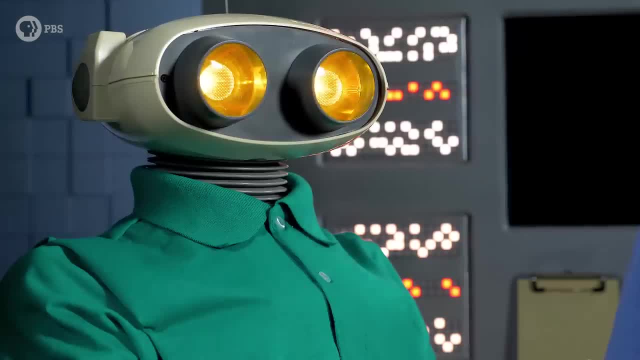 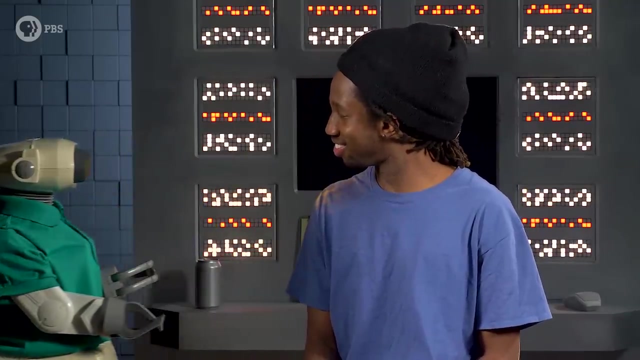 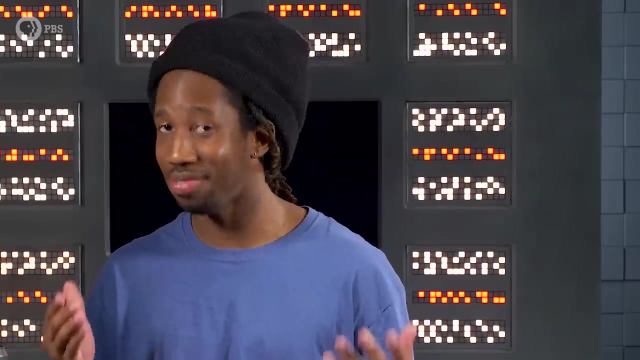 Which means John Greenbot should have a decision. Output neuron value: 0.93.. I believe that this is a dog. 93%. Hey, John Greenbot, nice job Thinking about how neural networks would process. just one image makes it clearer why AI needs. 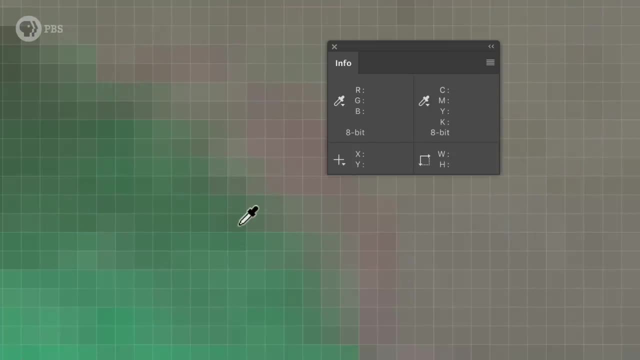 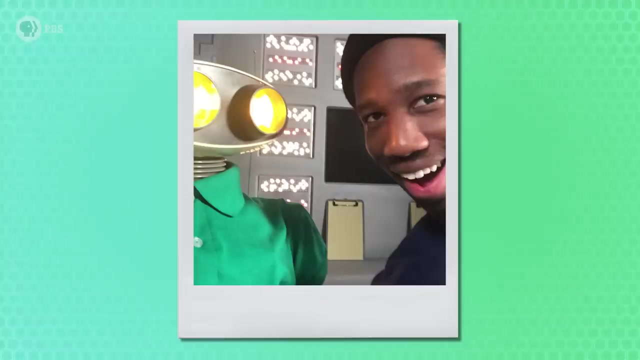 fast computers. Like I mentioned before, each pixel in a color image would be represented by three numbers – how much red, green and blue. it has So to process a thousand by a thousand pixel image, which in comparison is one pixel. 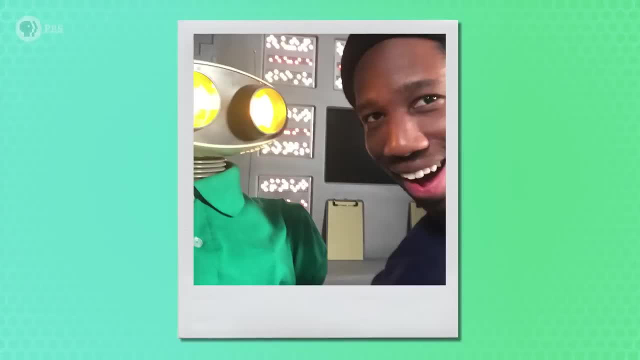 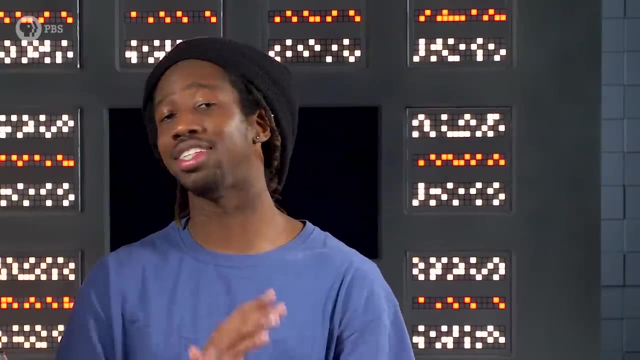 a neural network needs to look at 3 million features. AlexNet needed more than 60 million neurons to achieve this, which is a ton of math and could take a lot of time to compute, which is something we should keep in mind when designing. 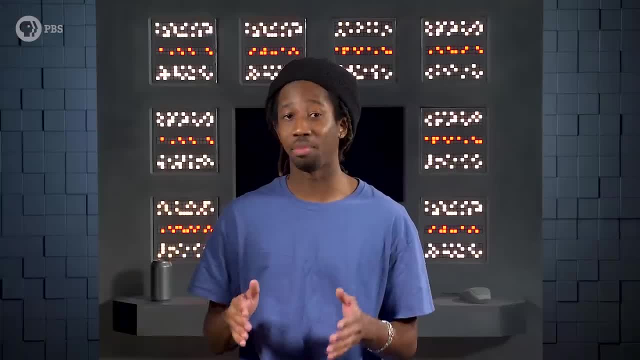 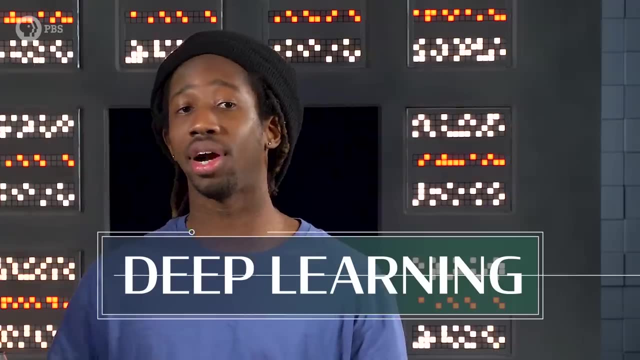 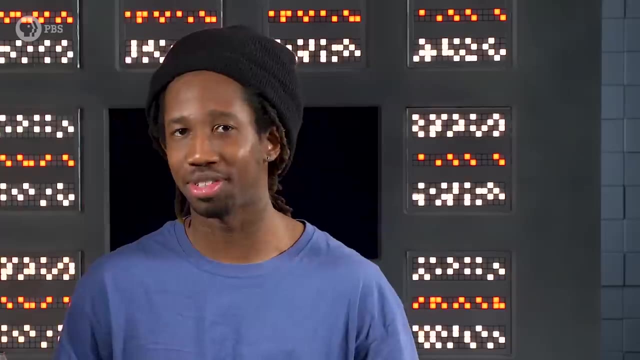 neural networks to solve problems. People are really excited about using deeper neural networks, which are networks with more hidden layers, to do deep learning. Deep networks can combine input data in more complex ways. So let's get started. First, we need to look for more complex components and solve trickier problems. But we can't make all networks like a billion layers deep, because more hidden layers means more math, which again would mean that we need faster computers. Plus, as a network gets deeper, it gets harder for us to make sense of why it's giving. 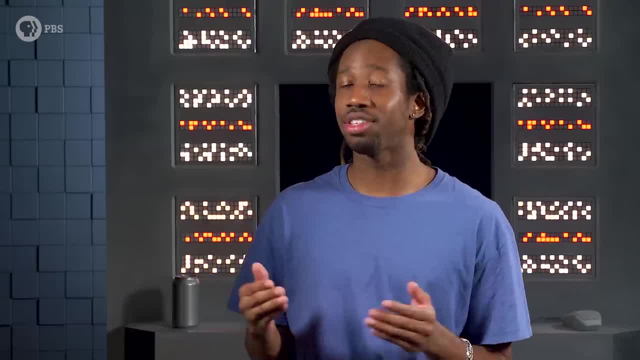 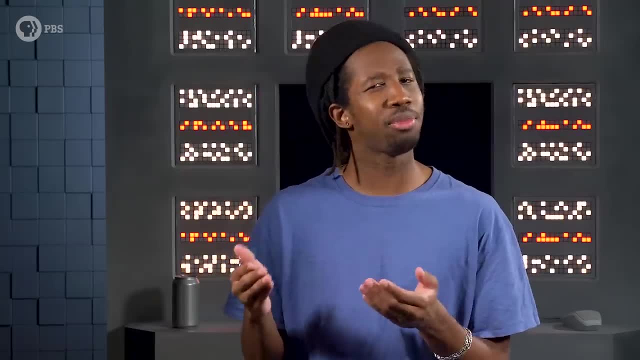 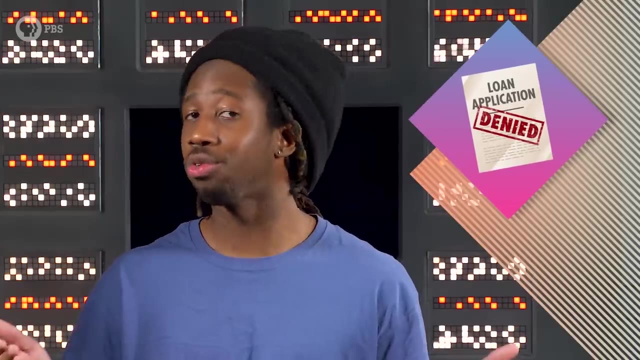 us the answers that it does. Each neuron in the first hidden layer is looking for some specific component of the input data, But in deeper layers those components get more abstract from how humans would describe the same data. Now this may not seem like a big deal, but if a neural network was used to deny our loan? 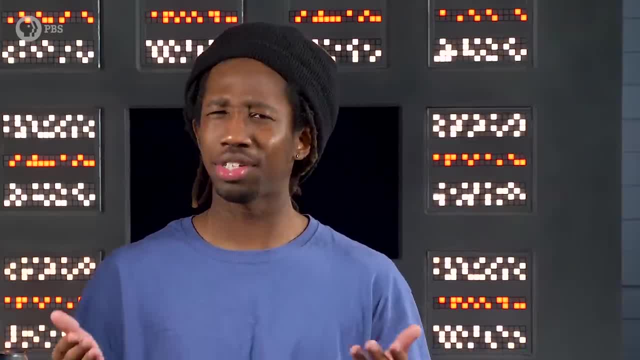 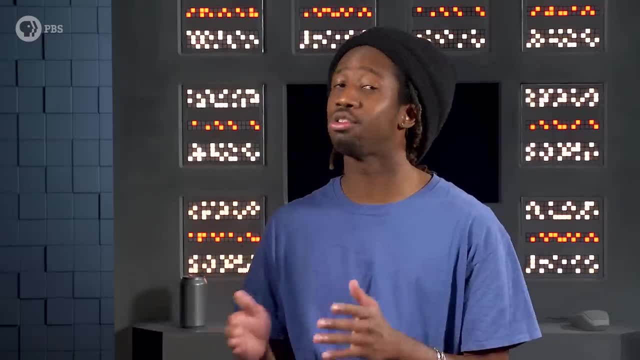 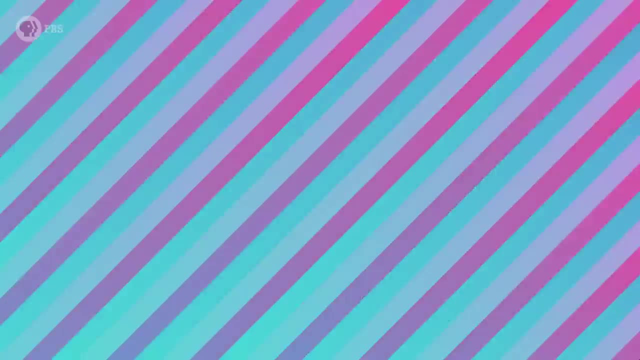 request. for example, we'd want to know why, Which features made the difference And how were they weighted towards the final answer? In many countries, we have the legal right to understand why these kinds of decisions were made, And neural networks are being used to make more and more decisions about our lives. 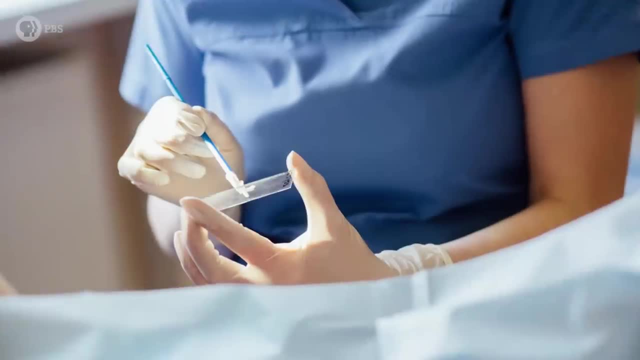 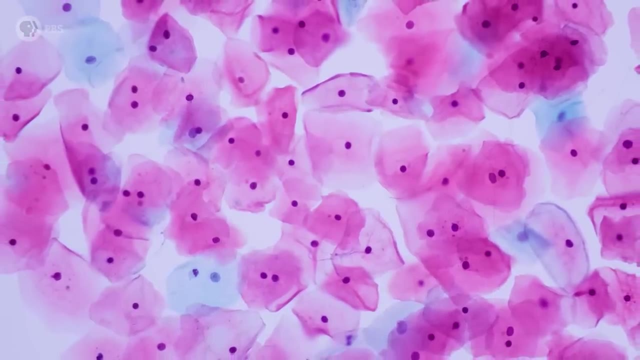 Most banks, for example, use neural networks to detect and prevent fraud. Many cancer tests, like the Pap test for cervical cancer, Use a neural network to look at an image of cells under a microscope and decide whether there's a risk of cancer. 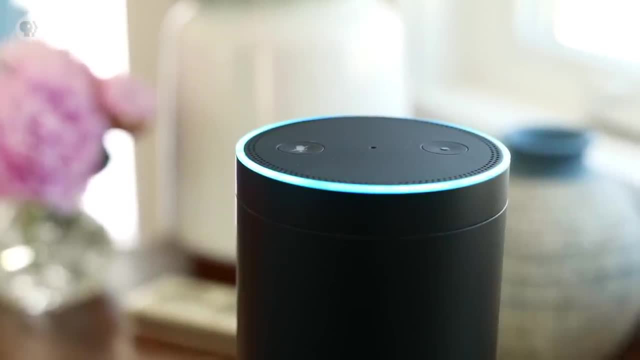 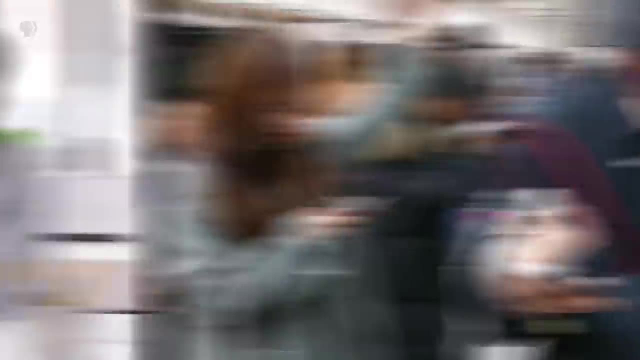 And neural networks are how Alexa understands what song you're asking her to play and how Facebook suggests tags for our photos. Understanding how all this happens is really important to being a human in the world right now, Whether or not you want to build your own neural network. 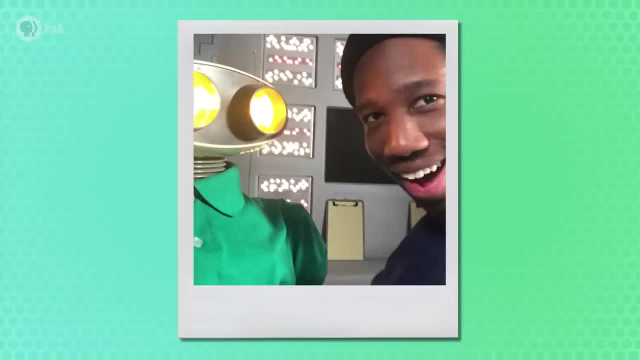 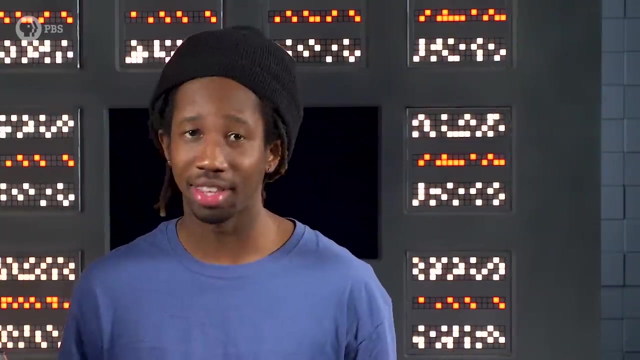 How much red, Green And blue it has. So to process a 1000x1000 pixel image, which in comparison is a small 3x3 photo, a neural network needs to look at 3 million features. AlexNet needed more than 60 million neurons to achieve this, which is a ton of math and 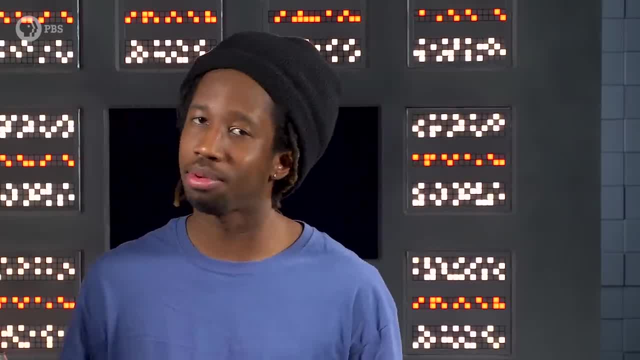 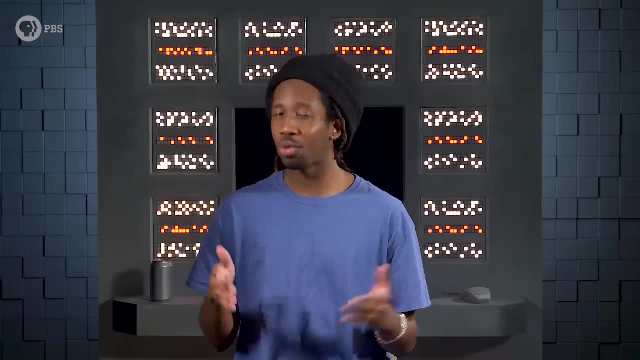 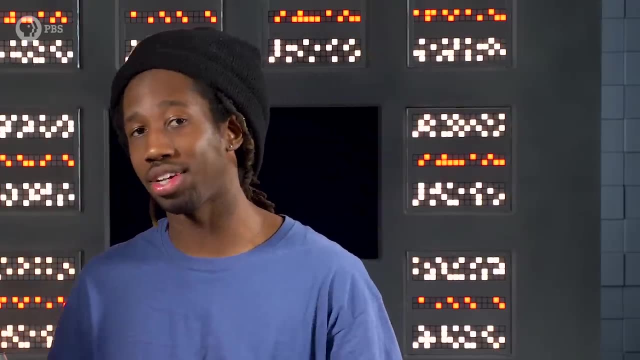 could take a lot of time to compute, which is something we should keep in mind when designing neural networks to solve problems. People are really excited about using deeper neural networks, which are networks with more hidden layers. Deep networks can combine input data in more complex ways to look for more complex components. 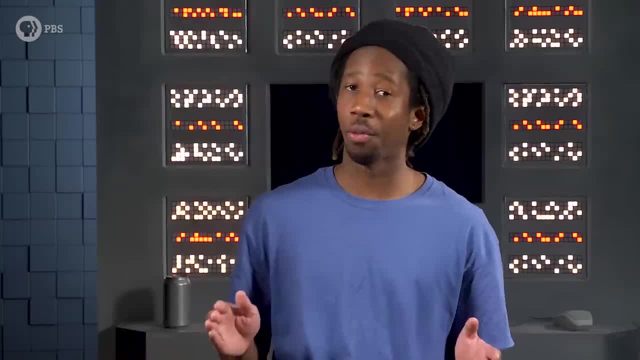 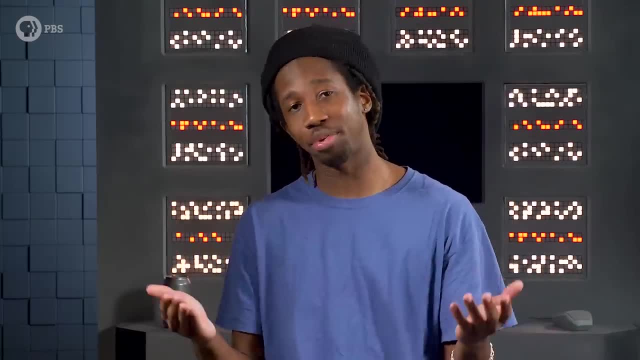 and solve trickier problems. But we can't make all networks like a billion layers deep, because more hidden layers means more math, which again would mean we need faster computers. Plus, as a network gets deeper, it gets harder for us to make sense of why it's giving. 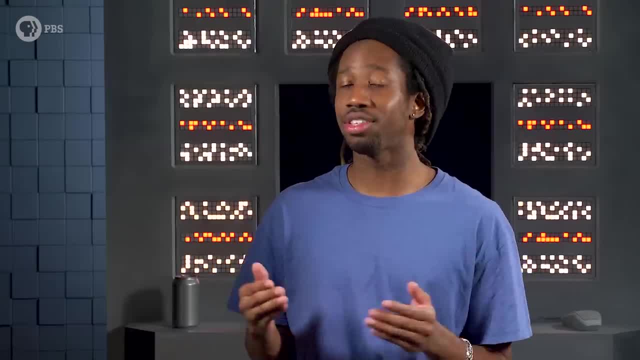 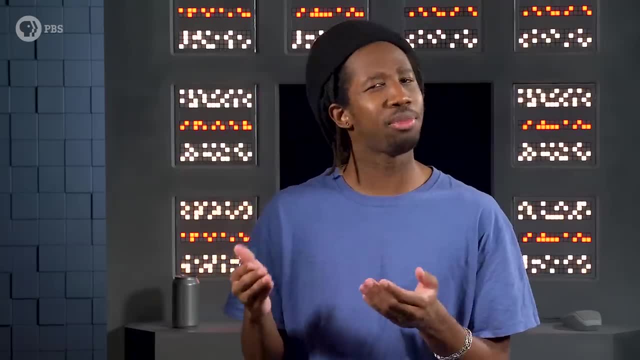 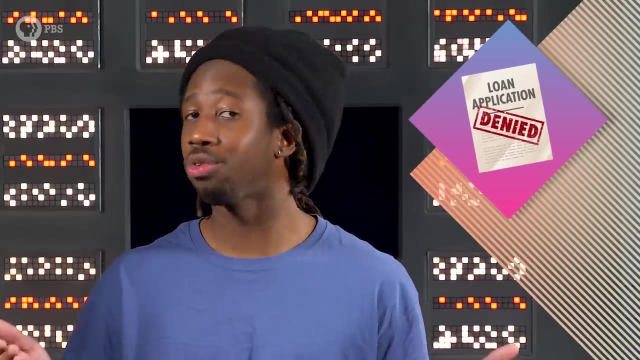 us the answers that it does. Each neuron in the first hidden layer is looking for some specific component of the input data, but in deeper layers those components get more abstract from how humans would describe the same data. Now this may not seem like a big deal, but if a neural network was used to deny our loan? 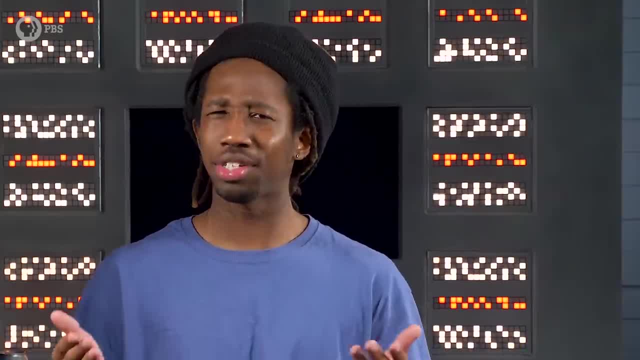 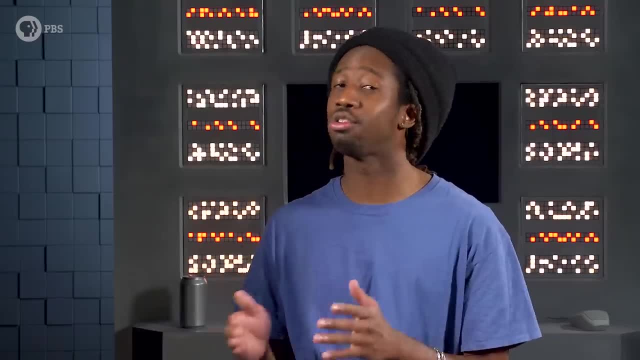 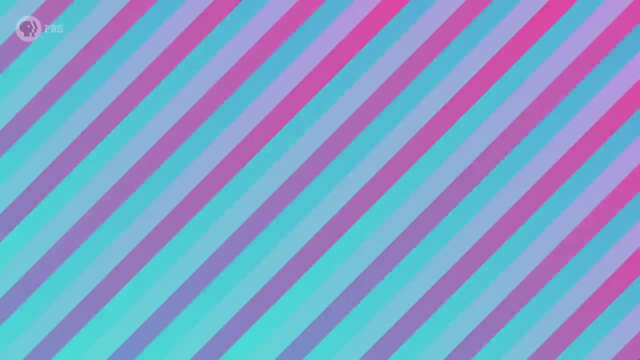 request. for example, we'd want to know why, Which features made the difference and how were they weighted towards the final answer? In many countries, we have the legal right to understand why these kinds of decisions were made, and neural networks are being used to make more and more decisions about our lives. 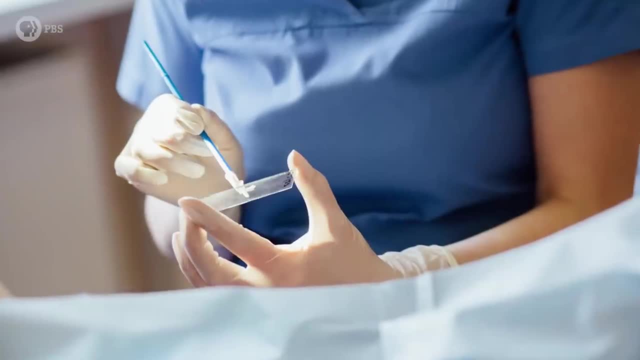 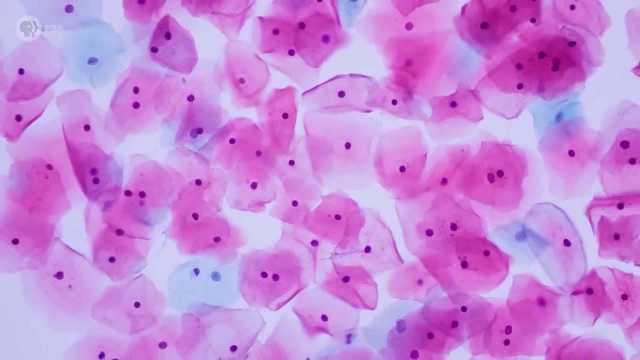 For example, use neural networks to detect and prevent fraud. Many cancer tests, like the Pap test for cervical cancer, use a neural network to look at an image of cells under a microscope and decide whether there's a risk of cancer. And neural networks are how Alexa understands what song you're asking her to play and 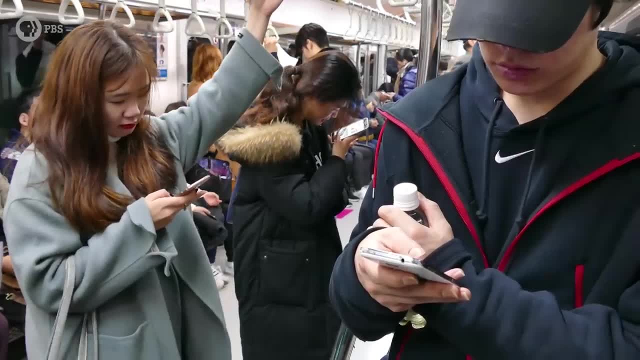 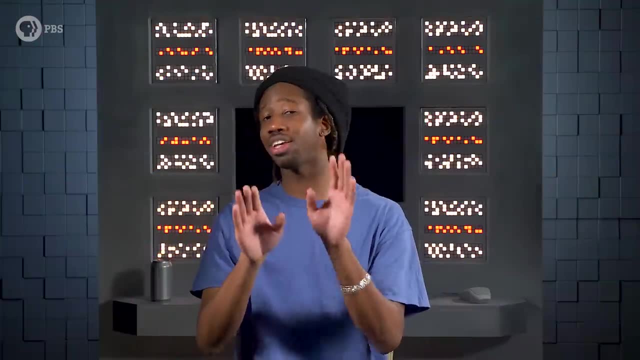 how Facebook suggests tags for our photos. Understanding how all this happens is really important to being a human in the world right now, Whether or not you want to build your own neural network. So this was a lot of big picture stuff, But the program we gave John Greenbot had a lot to do with it. 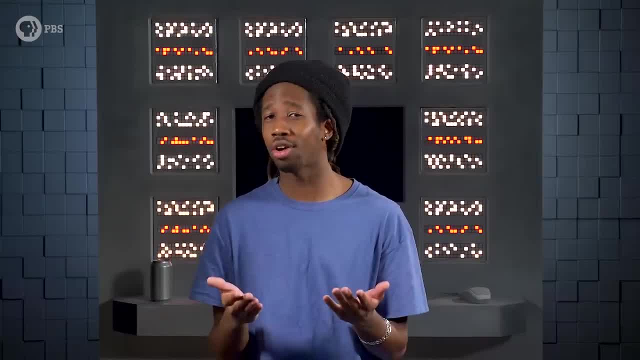